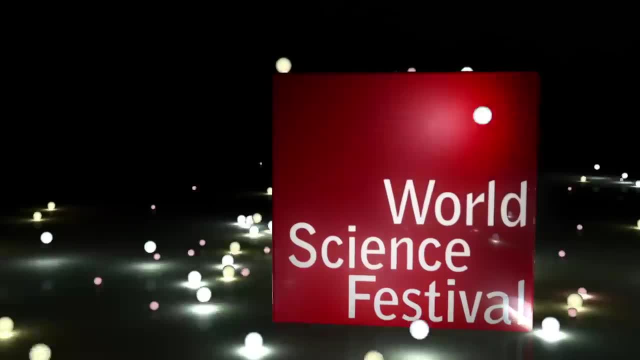 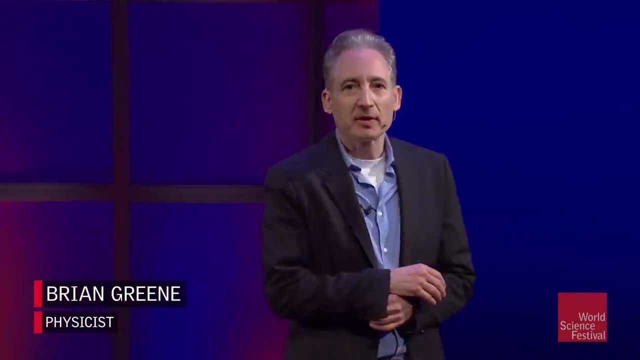 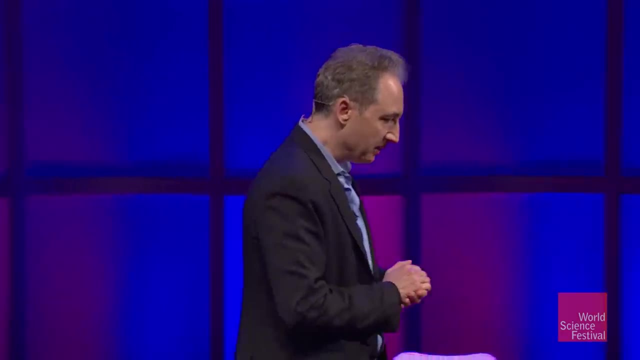 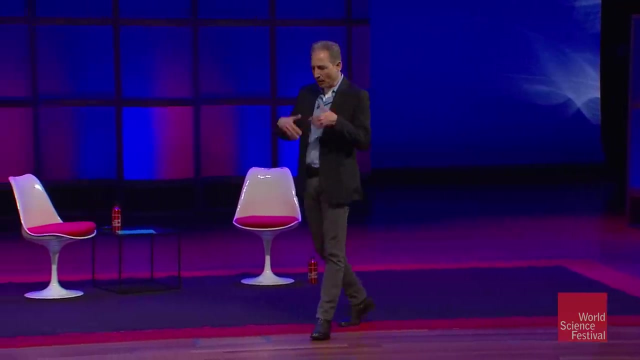 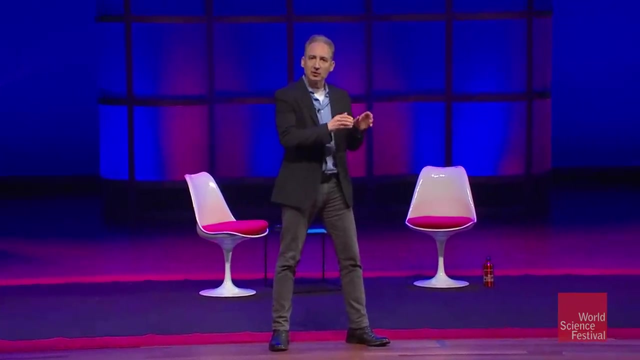 In talking about black holes, of course, Stephen Hawking is the great scientist who comes to mind, So I'd like to spend a little bit of time thinking about what it is that Hawking told us about black holes, what were the insights that he gave us, and what puzzles emerged from his work that we are still struggling to resolve. 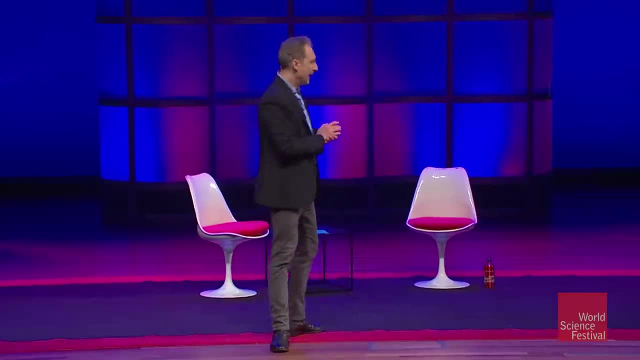 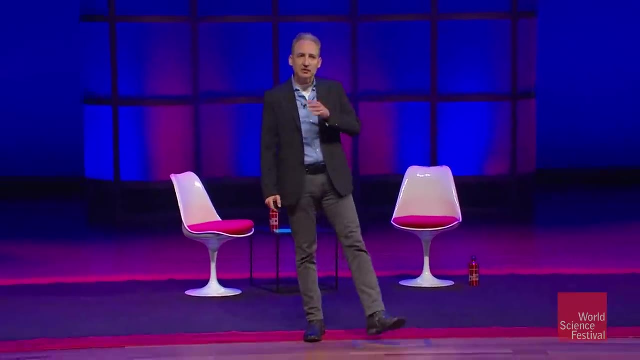 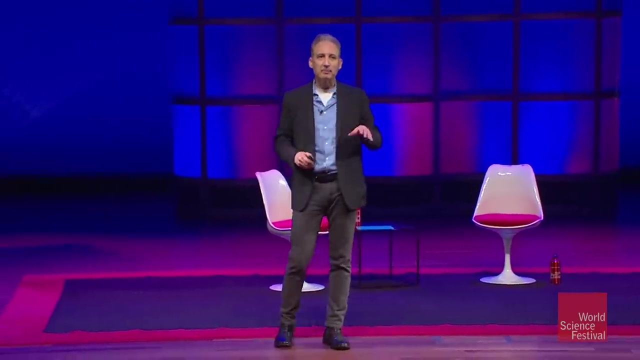 and probably will continue to struggle with for some time. And toward that end, as a little bit of background, we need to have some understanding of a concept that everybody is familiar with at some level or another, but let's use this opportunity to get us all in the same place. 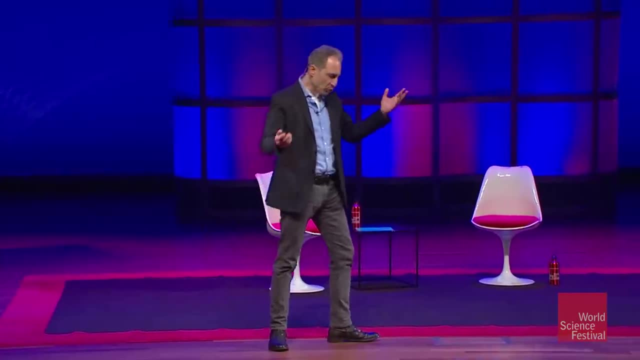 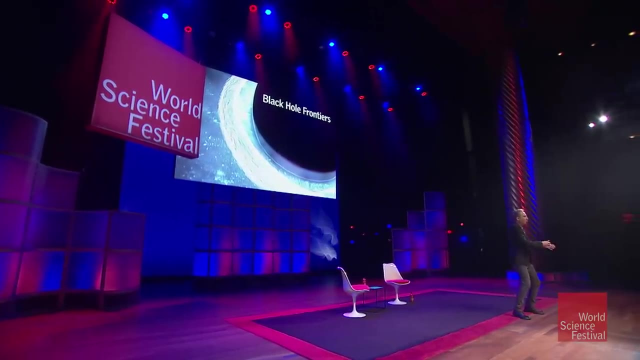 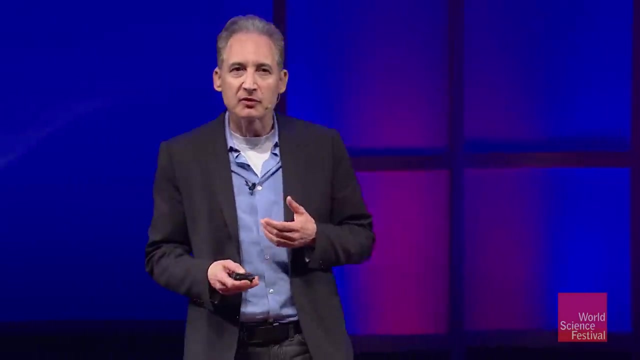 and that's the concept of entropy. So entropy is a word that's freely used in the culture. We often use it to describe a certain amount of going from order to disorder, That's, going from low entropy to high entropy. That's sort of the intuition that the culture has about this word. 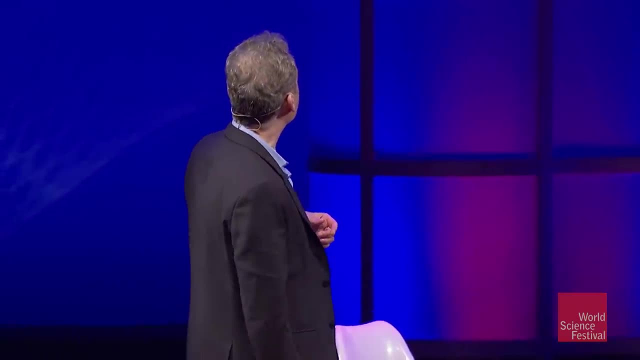 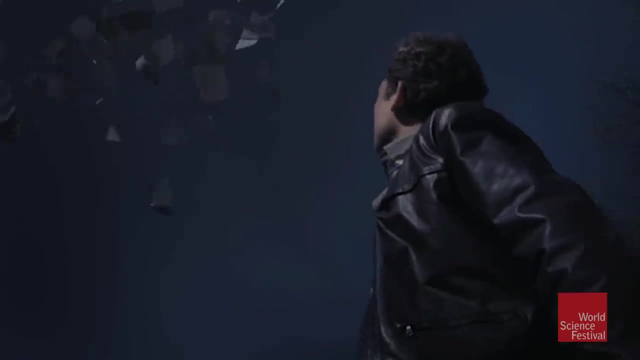 So let's start with that very basic way of thinking about entropy. And a good example would be: let's say I take my book, I throw it up in the air. it starts very ordered. All the pages were in complete numerical order. 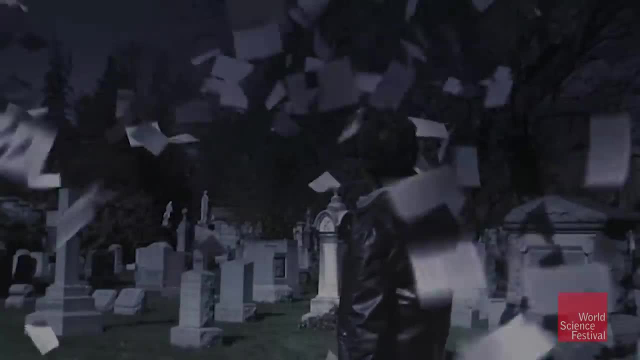 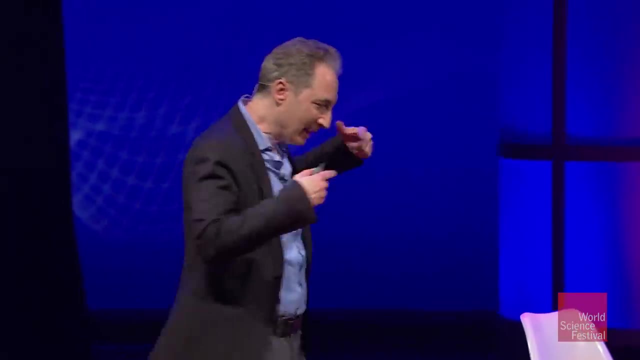 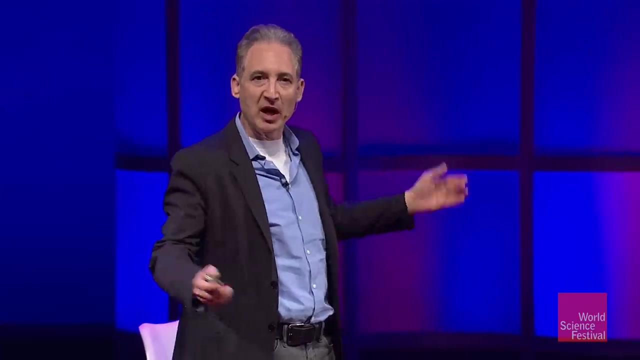 But as they come down, it's overwhelmingly likely that they will not land in numerical order. They'll land in a highly disordered state, And that gives you some sense of what it means to go from an ordered arrangement to a highly disordered arrangement. 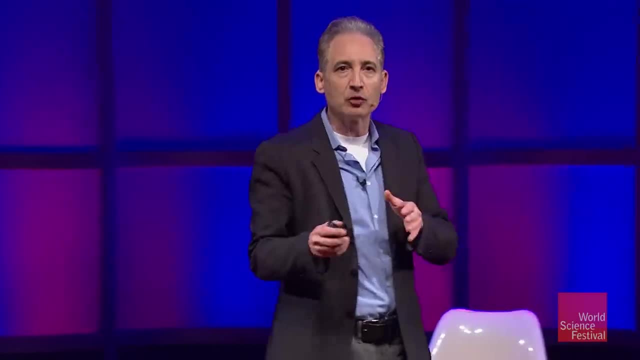 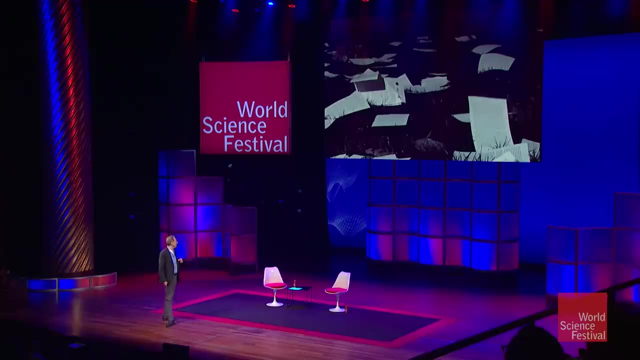 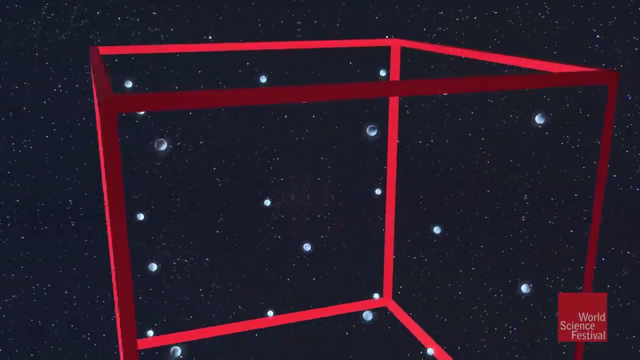 going from low entropy to higher entropy. Now, of course, that's just a sort of fanciful everyday example. If we head more toward a physics example, we could imagine having a a box of gas and imagine it just has a small number of atoms in there. 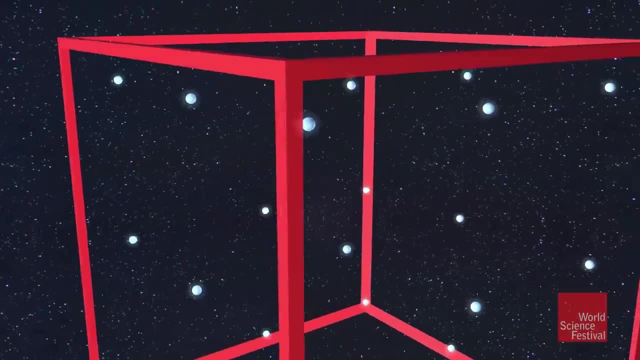 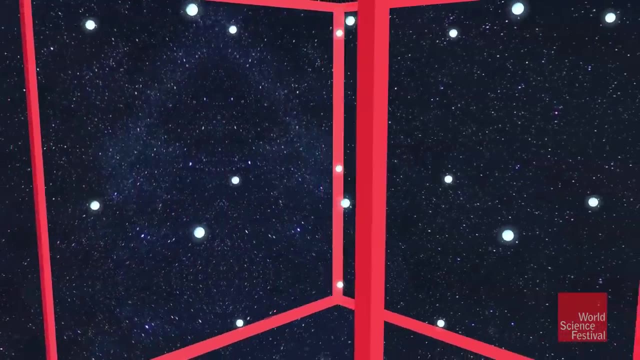 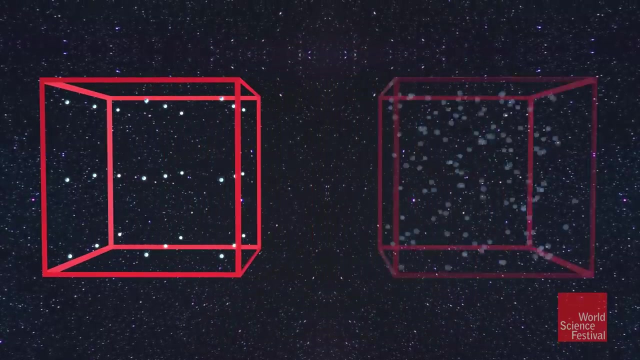 And imagine that they're all neatly arranged in this nice cubic lattice. This would be a very ordered or low entropy configuration of the gas, like the pages, all in numerical order. Now contrast that with a box of gas that has a whole lot of atoms. 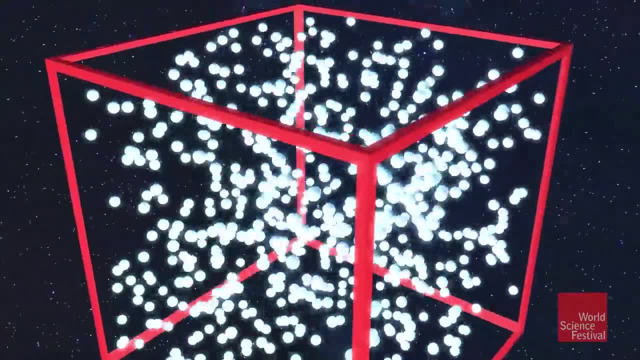 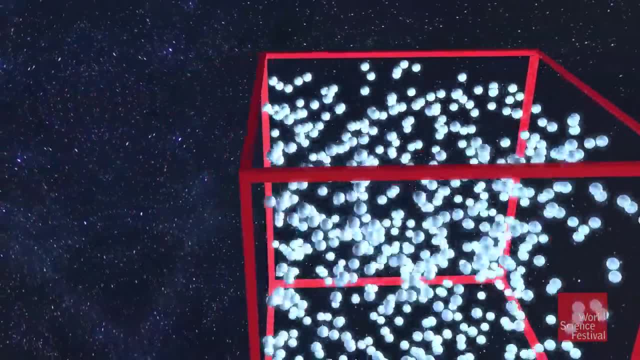 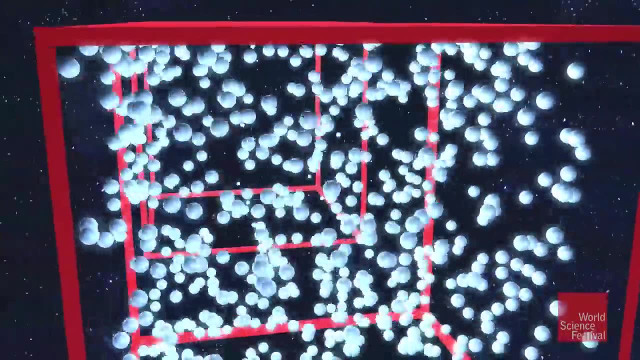 a whole lot of particles are all bouncing around in a completely haphazard way. This would be a very disordered state, a high entropy state, And another way of thinking about the distinction between low entropy and high entropy, which we'll be making use of in just a moment. 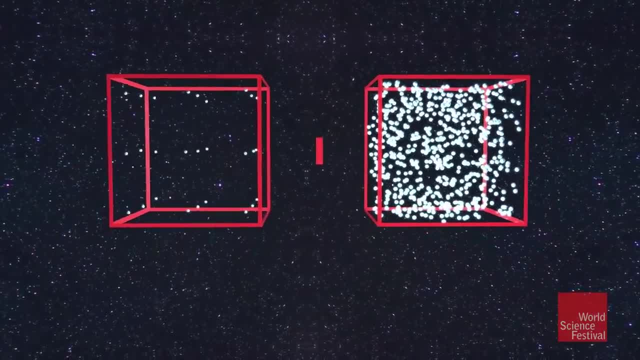 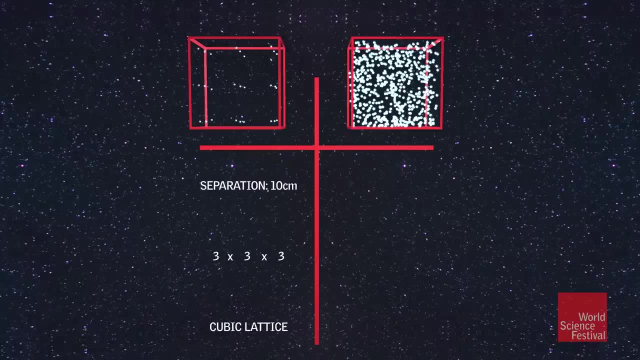 is the amount of information that would be required to describe these two configurations? Because, look on the left, you don't need a lot of data. It's a cubic lattice. You've got three by three, by three atoms filling out that lattice. 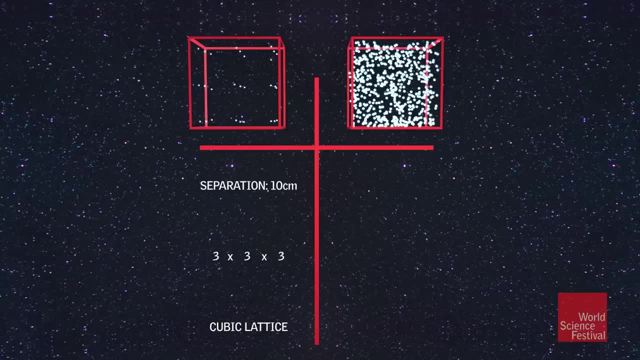 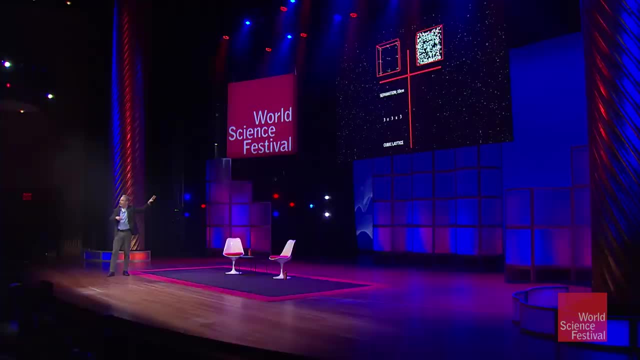 And if I give you the separation of them, say 10 centimeters, that basically describes the configuration on the left. You don't need a lot of information to describe a system that has low entropy. But let's say I wanted to describe the configuration on the right. 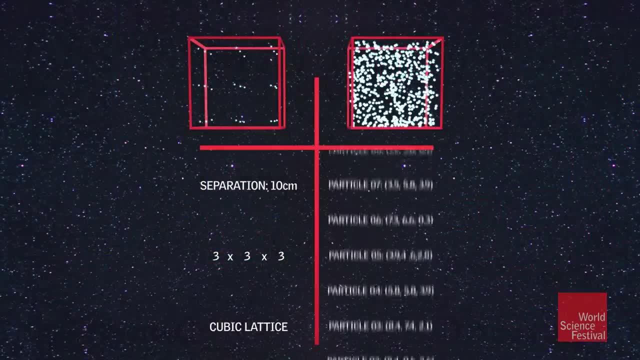 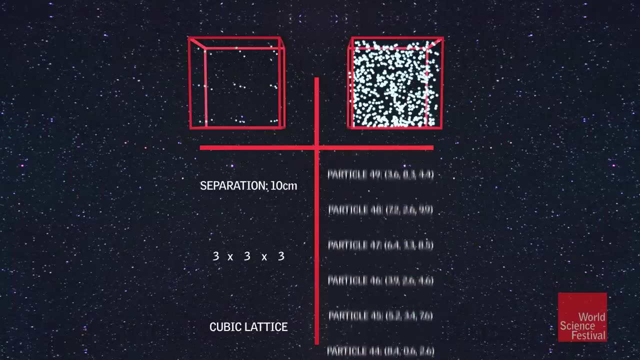 Well, I basically have to tell you where each and every particle is located. That's the only way I could describe it. Look at all the information I need to describe that configuration. So the idea is low entropy, not a lot of information. 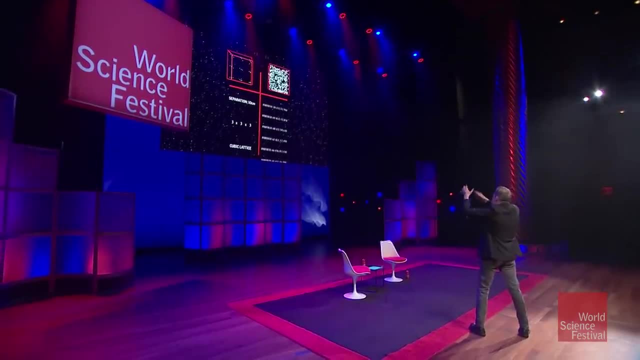 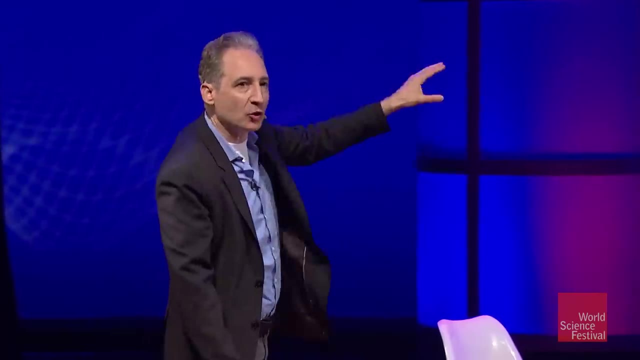 high entropy takes a lot of information that's hidden in this configuration of particles And that's kind of the distinction between order disorder: low entropy, high entropy, low information, high information. Now, of course I'm talking in loose language. 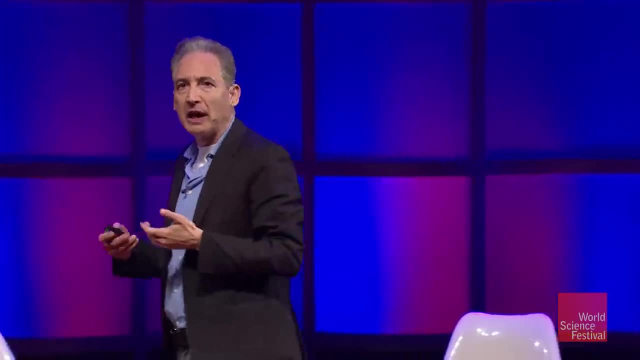 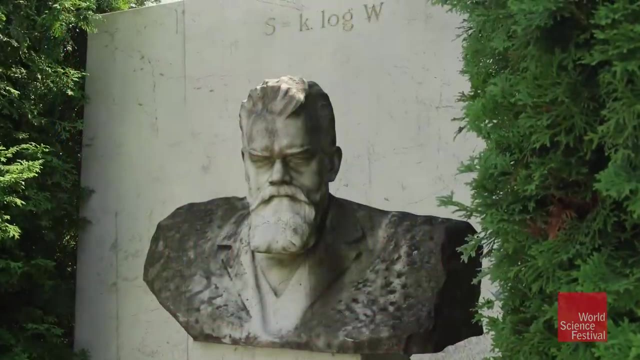 so that we can all get a feel for the critical ideas. But you can make this all quite precise. And this gentleman over here, you know who this is. Who's this? Ludwig Boltzmann, that's right, And this is his famous tombstone. 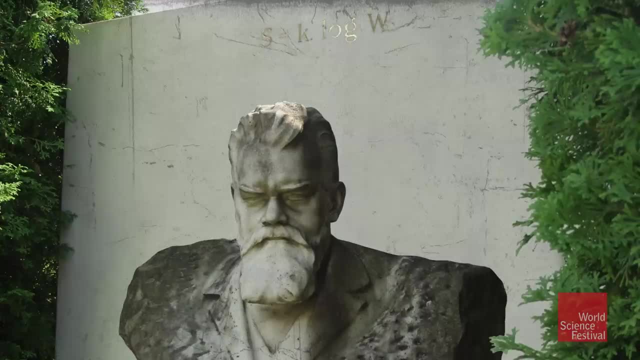 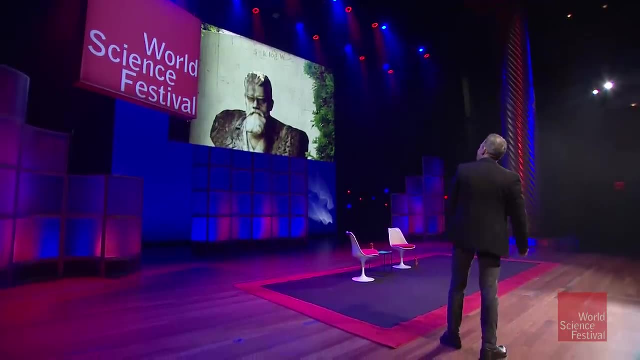 And you see that formula on the top of his tombstone. And that is the formula that makes these statements precise. This is a formula that you learn if you take a course in statistical mechanics. thermodynamics: S stands for entropy, K is Boltzmann's constant. 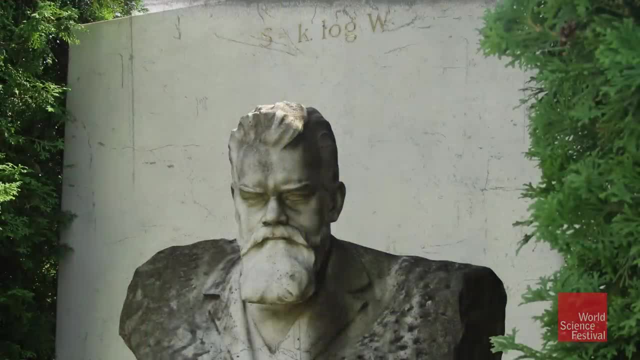 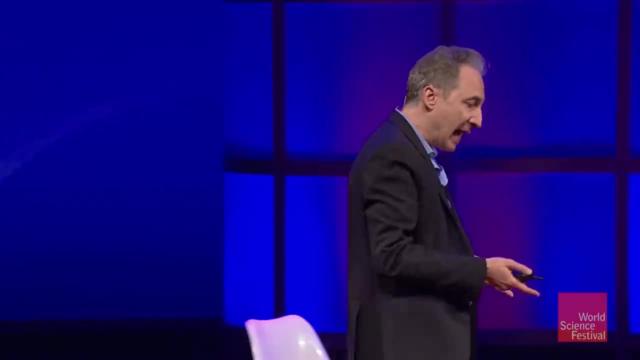 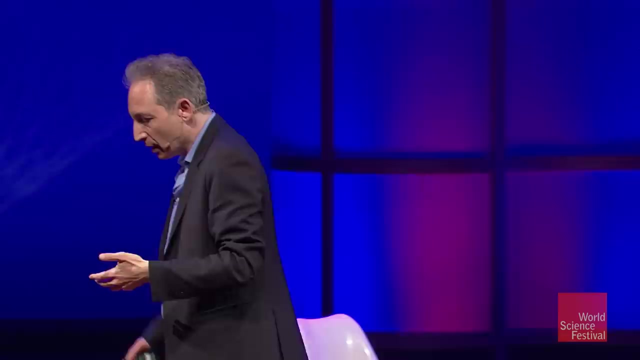 and the rest of it has to do with the number of configuration of the ingredients, of the particles that make up the system, And the famous second law of thermodynamics makes use of this formula And again, it's something that we're quite familiar with in the culture. 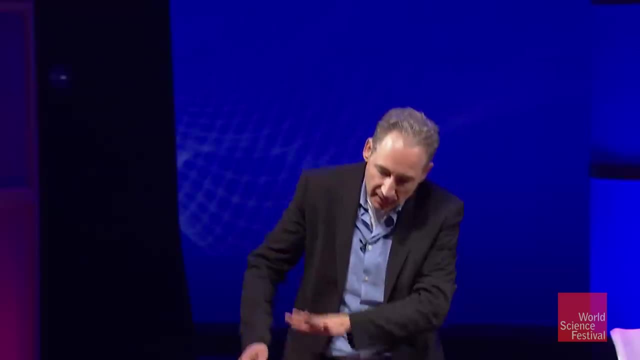 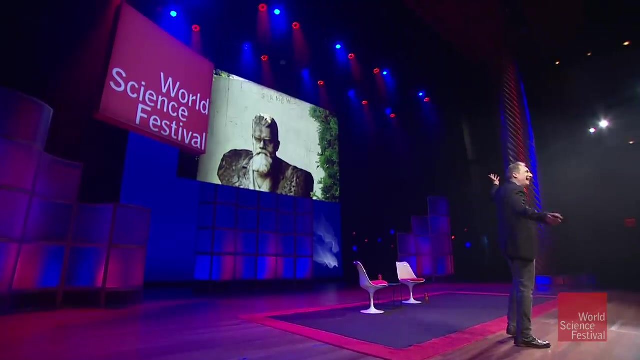 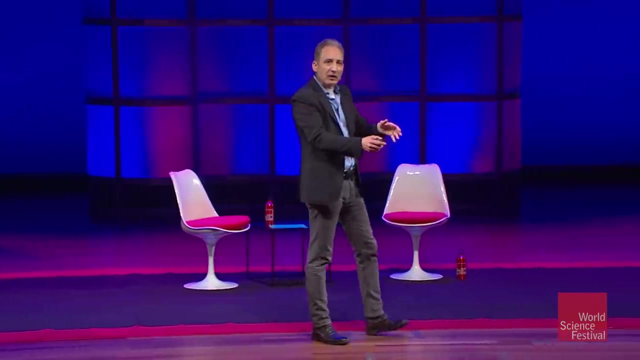 that things typically go, as I said, from low entropy to high. That's the natural progression of a system, which means that this quantity S tends to increase over time. The entropy later on is almost always greater than the entropy earlier on In the evolution of a system. 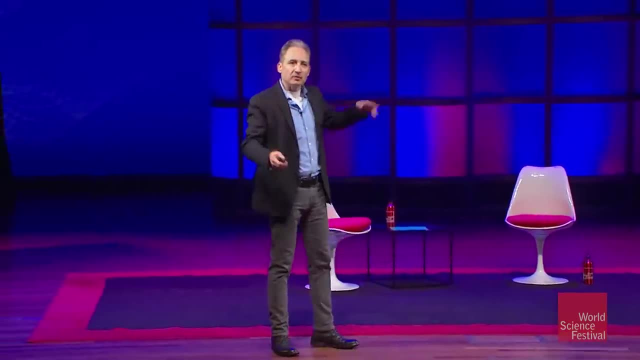 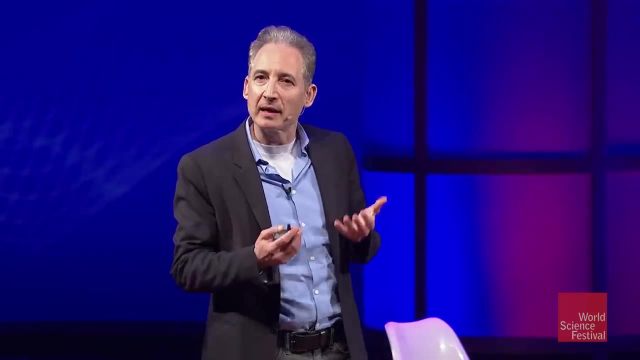 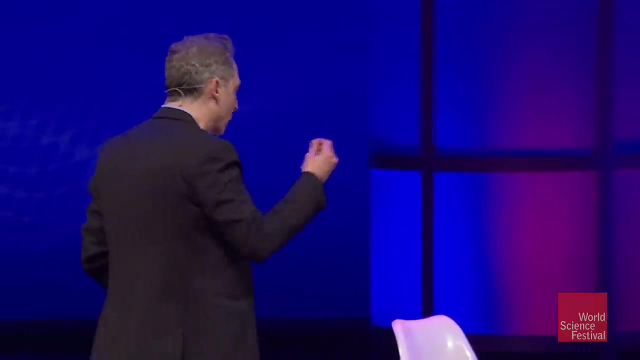 And what we'd like to do now is have this idea come into contact with the idea of black holes And we'll see that there's a certain kind of tension that arises. It's a very fruitful tension that will take our understanding further as we try to come to grips with it. 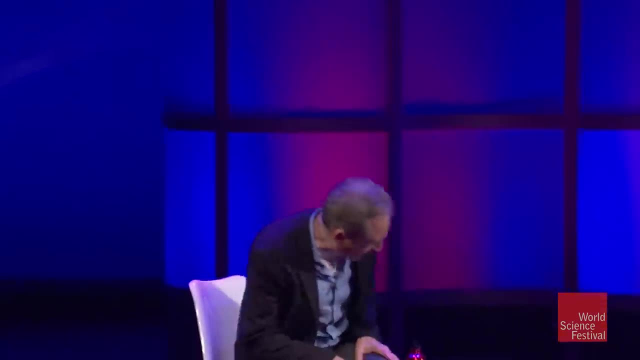 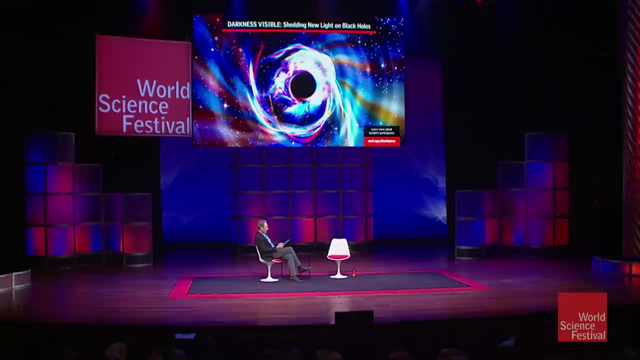 And to help us go on that journey, we're going to now bring out the Donner, Professor of Science in the Department of Physics at Harvard, whose primary area of research is string theory. He's received numerous awards and recognitions for his work. 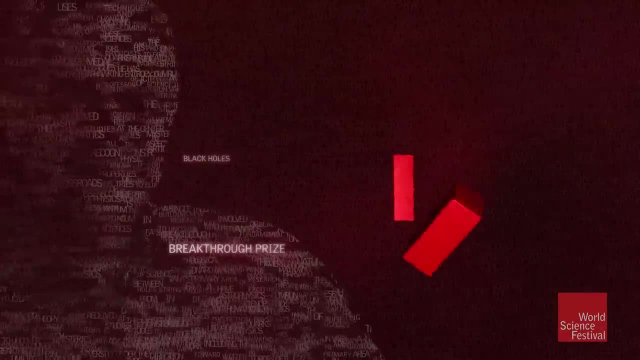 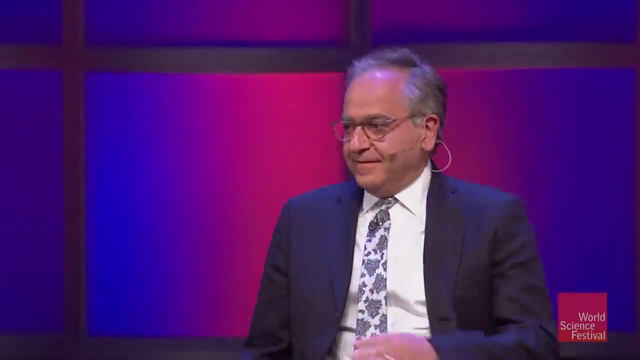 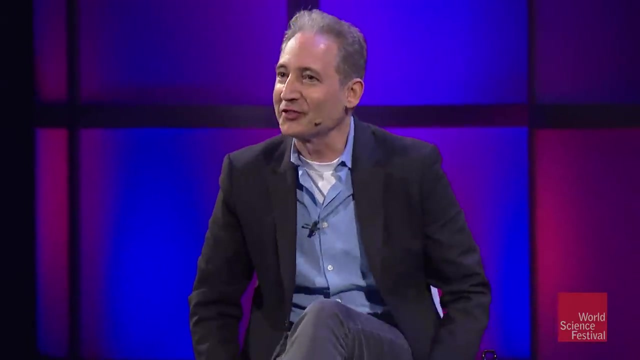 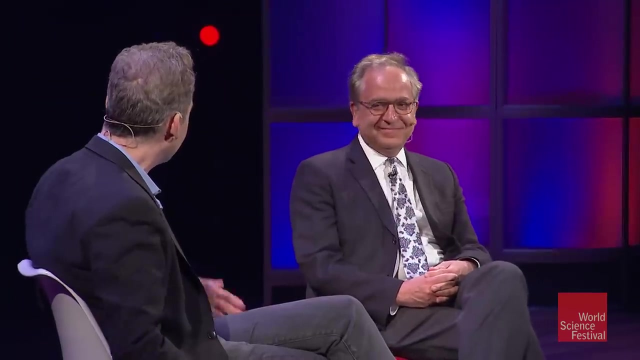 including the Dirac Medal and the Breakthrough Prize. Please welcome Kumrun Vafa. Now, I should say that I have known this gentleman for over 30 years. We were, I guess, both postdocs At Harvard in the 1980s. 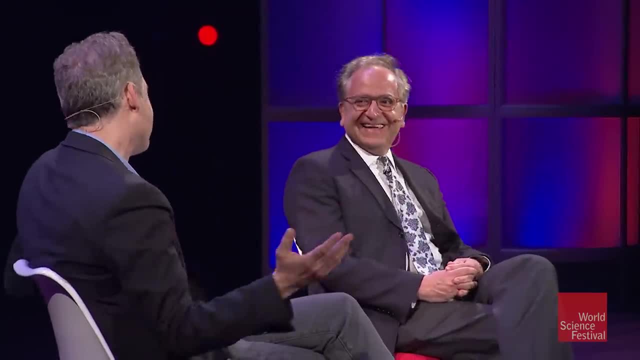 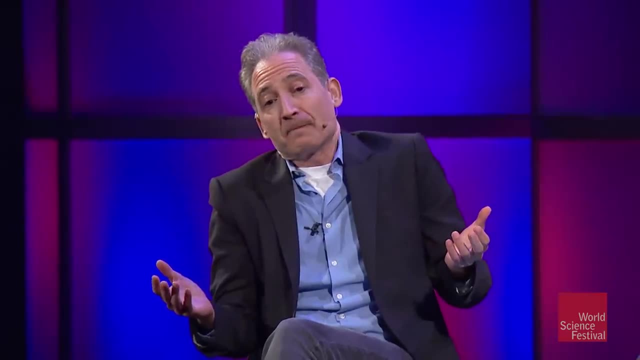 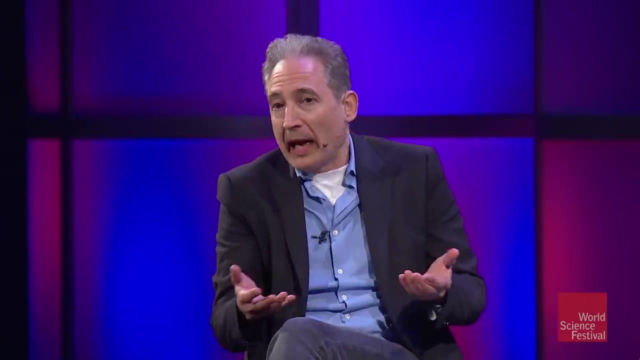 That's right. You got a job at Harvard as faculty, But that's okay, We're still a good You're doing very well, Thank you, And I should say my most exciting intellectual adventures in string theory have been the papers that we have done together. 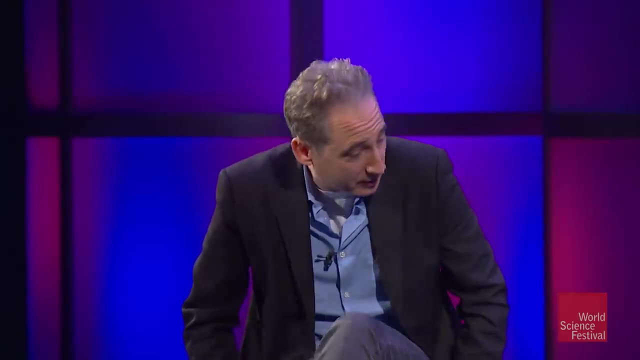 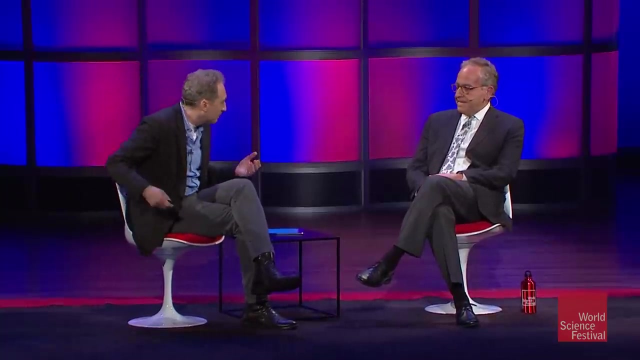 Thank you. We had a lot of fun with you, Brian, Thank you. So it's been an honor to work with you, So thank you, Thank you. So let's get into this subject here. We heard a little bit about entropy. 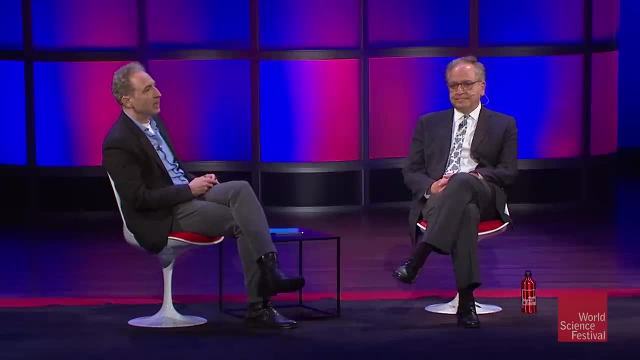 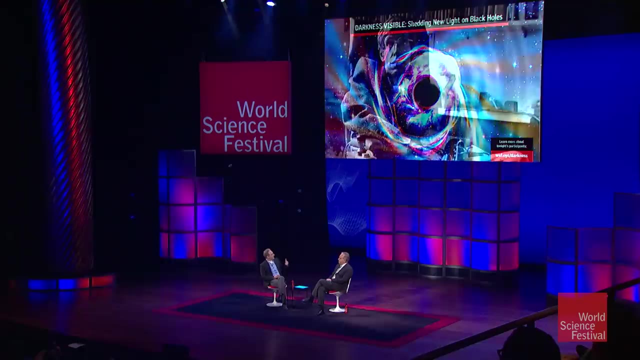 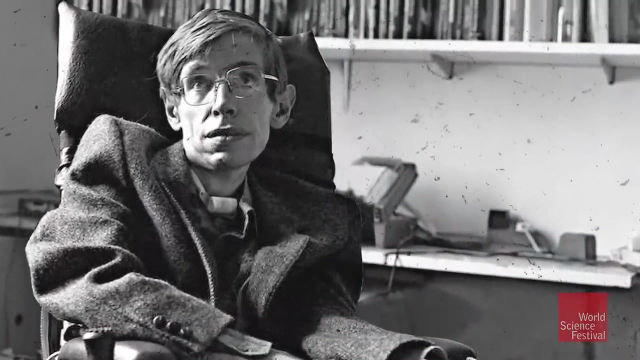 and about the second law, that entropy increases over time. But in the 1970s, people like Bekenstein and Hawking. they began to worry about how the second law of thermodynamics would behave in the environment of a black hole. So give us a sense of what they were puzzling about. 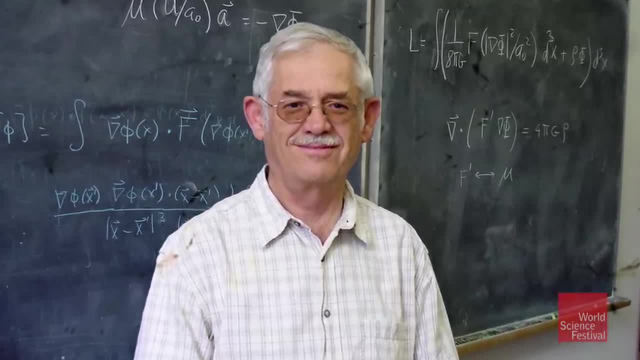 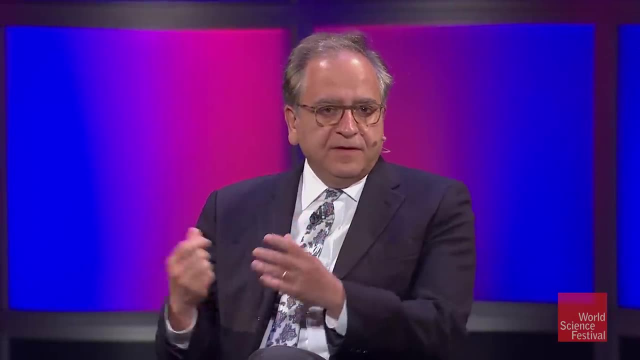 So part of the puzzle was the objects they knew would fall into the black holes, but they cannot come out. So objects that are falling in have entropy, just like what Brian already described. You have some information about where they are or how they are. 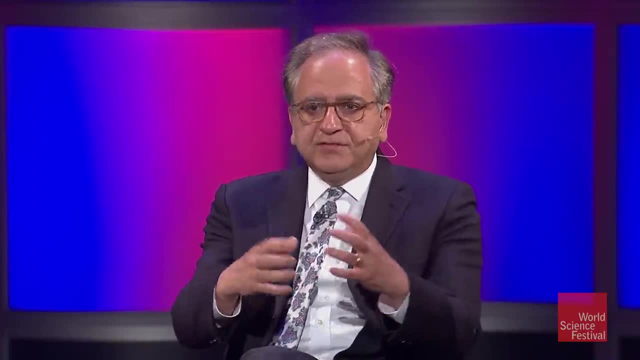 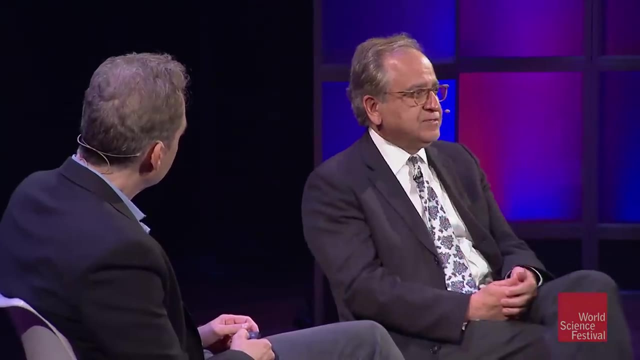 But once you fall into the black hole, then you don't have any more access to that information. So what happened to that information? So that seems like you lost entropy. Entropy went down, and that's against what Boltzmann said. 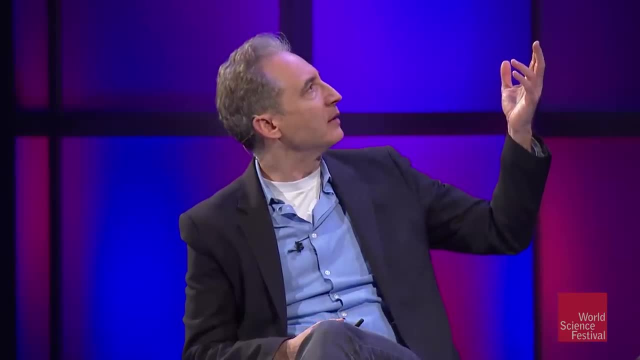 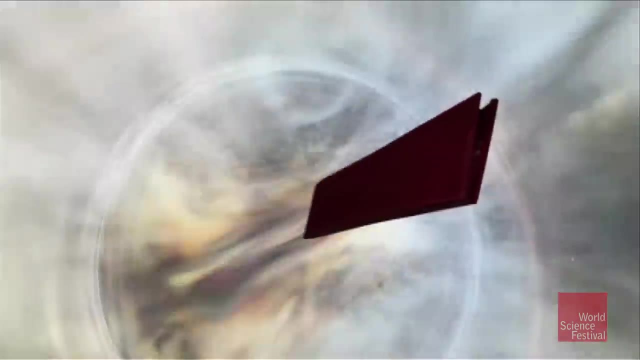 So can I give a concrete example of that? So I think we have a little silly example. If I took my wallet, it has information, It has entropy. I throw it into the black hole and you're asking what happened to that entropy. 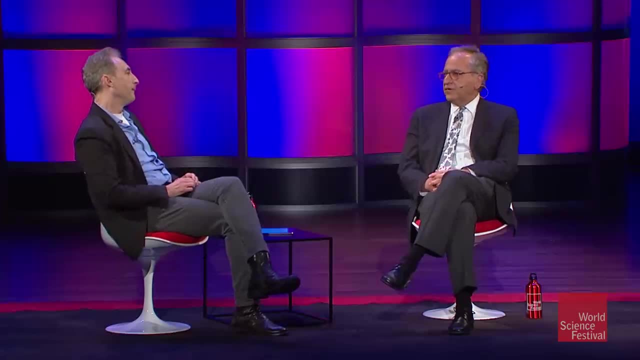 Did it disappear from the universe Exactly? So that was the kind of question that they were struggling to understand: How could this be consistent, Right? So they began thinking about this, and then there were a few ideas that they were thinking about. 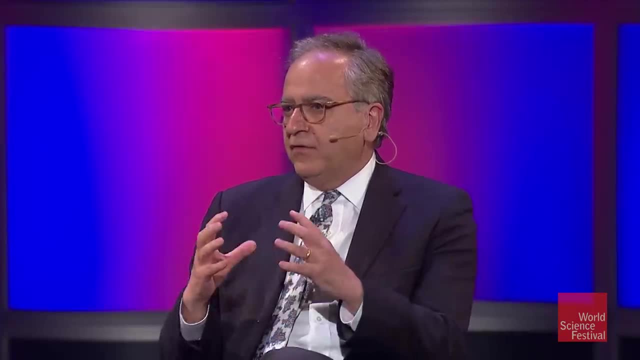 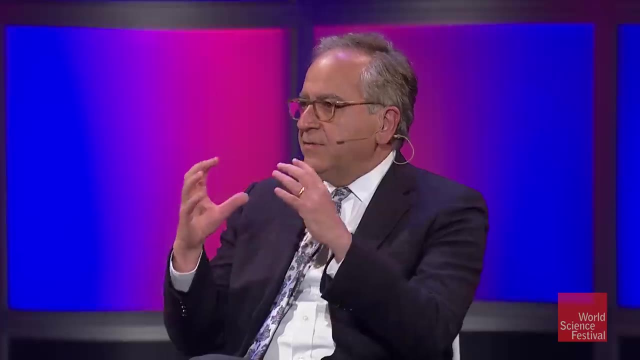 and, in particular, the properties of the horizon of a black hole, The edge, The edge, The event horizon that we talked about, The edge Beyond which no light can escape. They found it had some interesting properties and, in particular, they began studying what is the area. 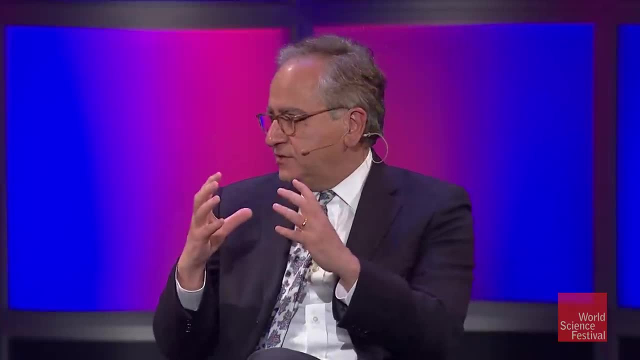 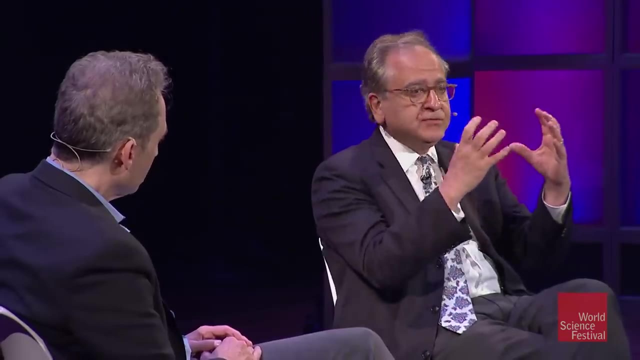 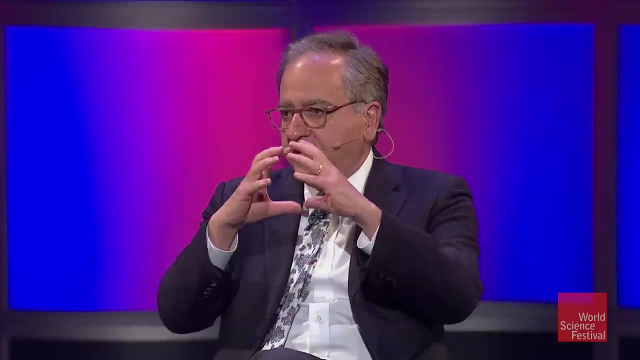 What is the area of this edge And how does it change? And, in particular, what happens if you throw objects into this black hole? What happens to this area? Yeah, And one of the surprising things they found was that when you throw objects in this area cannot stay put. 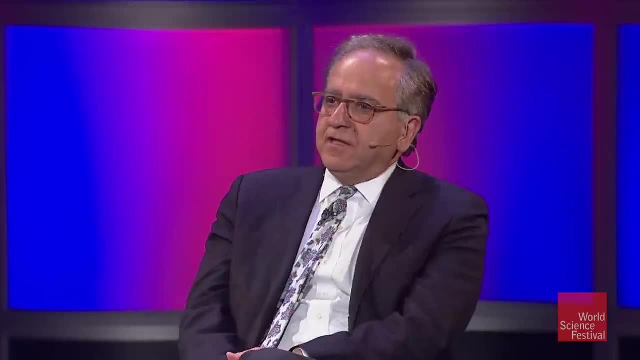 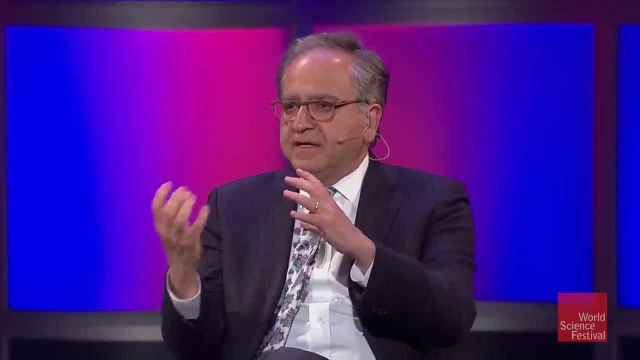 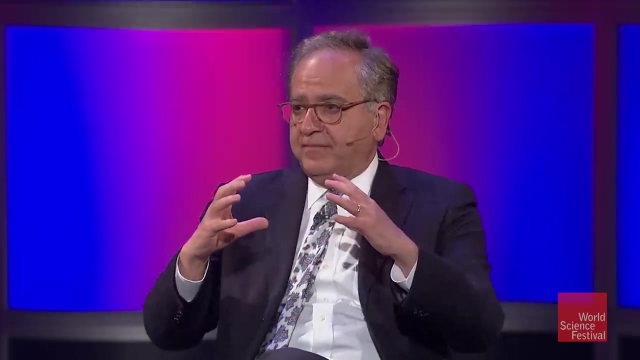 and, in fact, increases Yep. So they began to think about: okay, what could this mean about this? what this could be related in some way compensated by the fact that you're losing something, the entropy- Could it be somehow compensated by the fact that this area is growing? 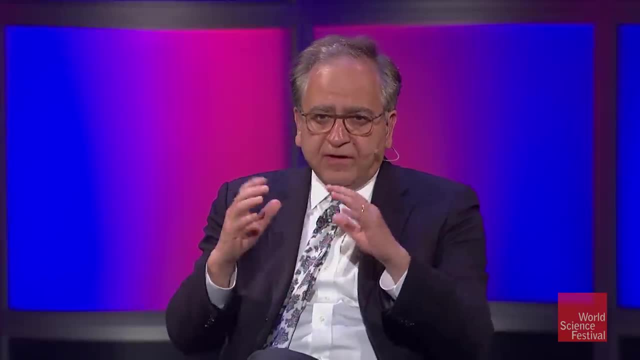 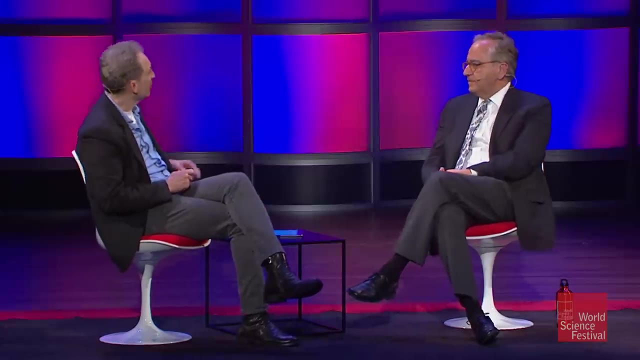 So they begin to ask the question: could the area of this event horizon be in any way related to the lost entropy? So we actually can unpack that. So let's just go through a couple of little examples here. So this is the standard second law of thermodynamics. 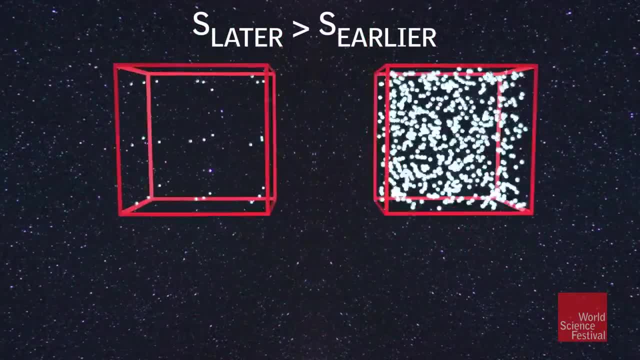 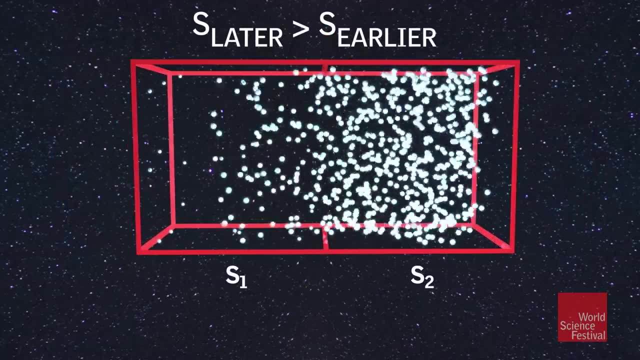 that entropy grows over time. Let's just take the two boxes that I started with to illustrate what you're describing. If we take those two boxes and we put them together, what happens to the entropy? It goes up right. That's the Boltzmann's thing. 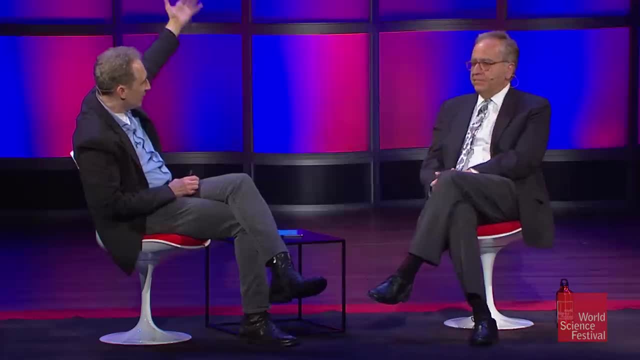 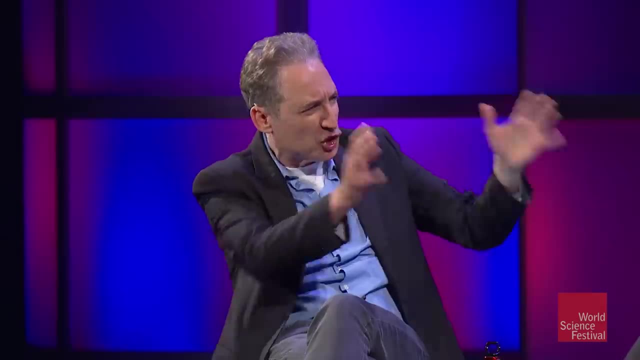 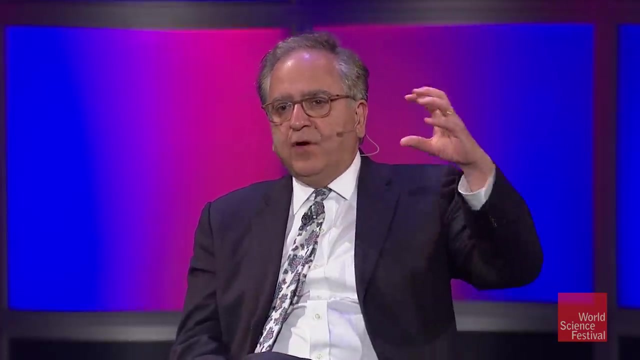 Right. So we have: the combined entropy is greater than the individual's entropy. Now you're describing something that doesn't have to do with gas in a box. You're talking about the geometry of a black hole. So, for example, they studied what happens if you study one black hole. 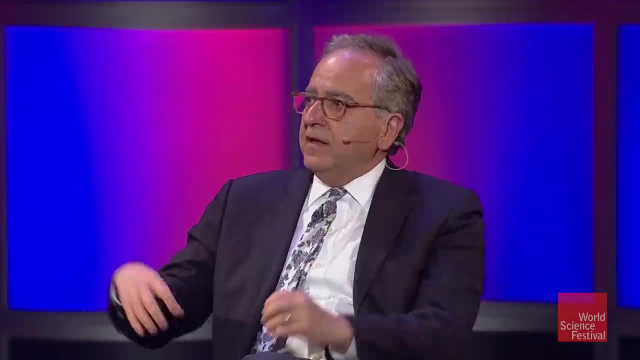 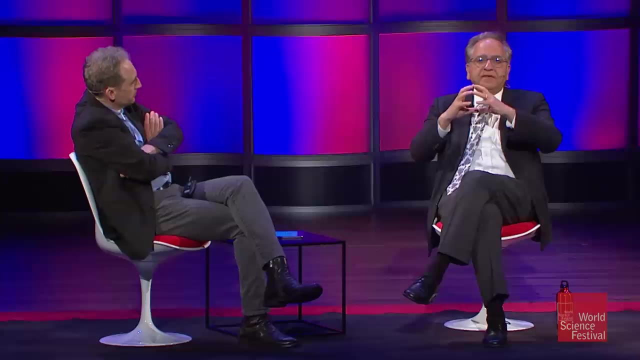 with one area of event horizon and another black hole with a different area, and you bring them together, you merge them and you get a new black hole with a new area, And they found that the area of the new formed black hole is bigger than the sum of the two areas. 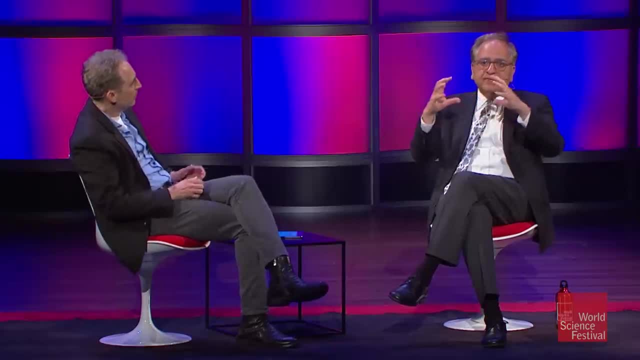 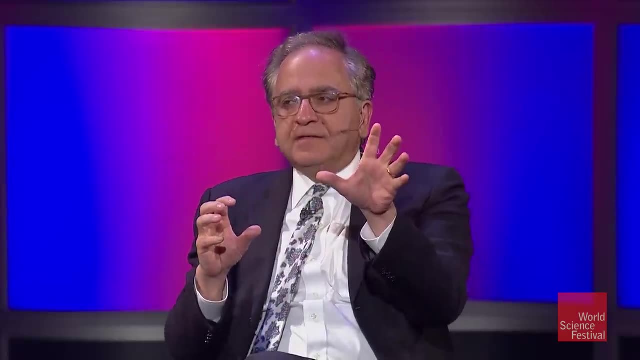 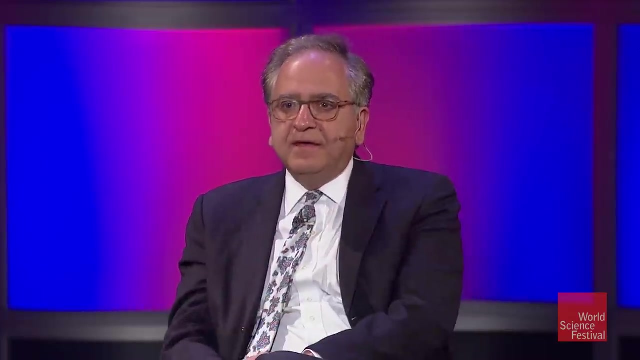 Just like the entropy had that property, the entropy resulting on the box, when you combine them, was bigger than the individual's entropy. So the entropy sounded very similar to the area, or area sounded very similar to the entropy. So they began asking: could it be that the area and the entropy are proportional? 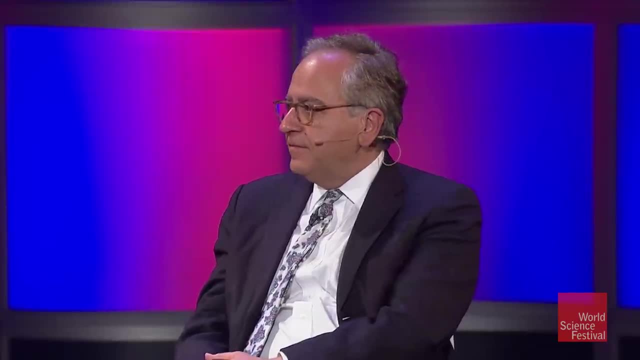 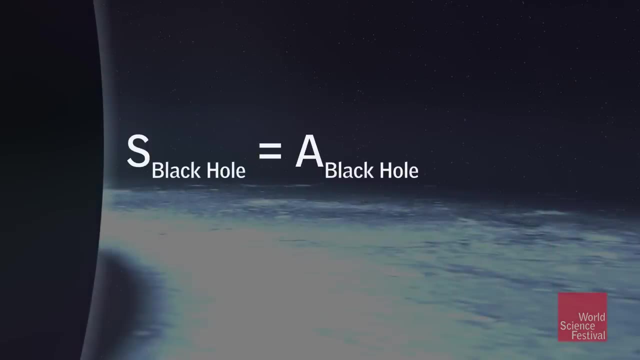 to one another for black holes, And indeed they found a formula that we can bring up here. So entropy is the area and the proportionality constant is a little bit complicated, But you don't really have to worry too much about that. 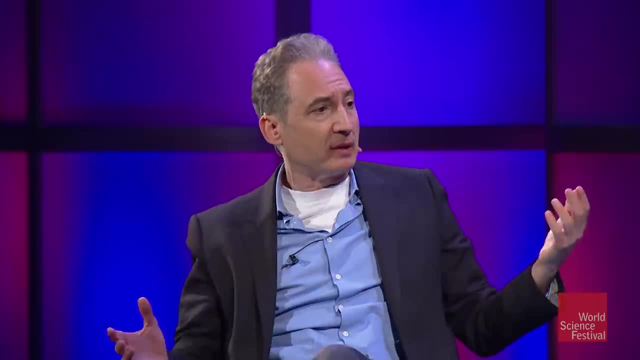 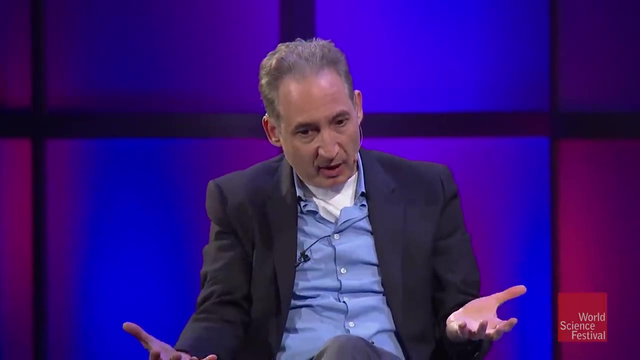 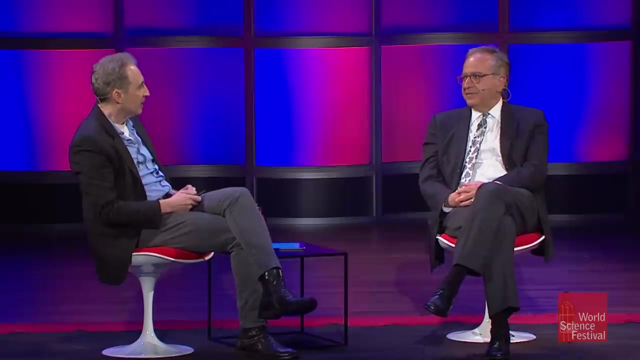 This number on the right-hand side. But the basic lesson is that they're guessing. they're suggesting that the area of the event horizon is somehow holding on to the entropy, holding on to the information. in some sense, that's inside the black hole. 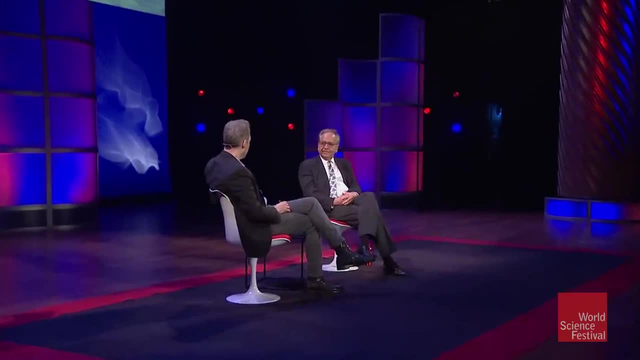 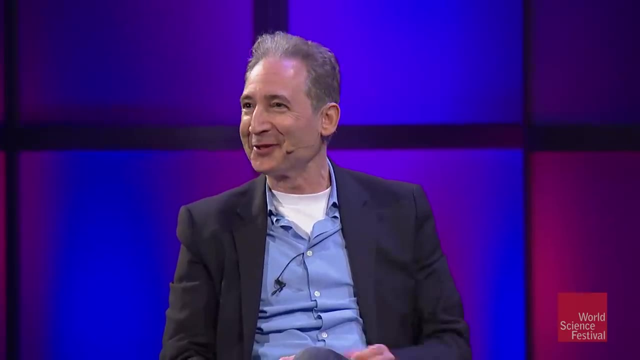 Now you gave an interesting thought experiment about how to test that. You were talking about throwing something in and watching the area, And it just so happens that we have a little sick man Accident Accident on that here, So why don't we go through that? 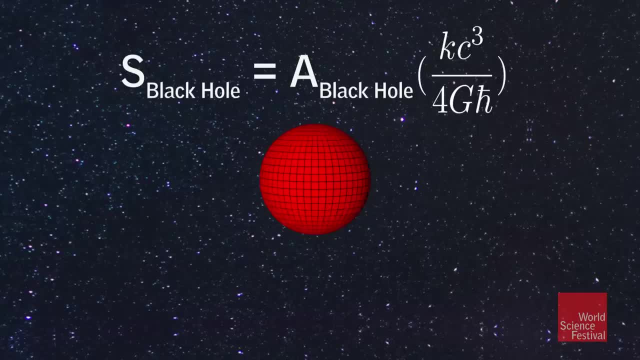 So what are we seeing here? And then we'll do your little thought experiment. So here, I guess, we are seeing a black hole, a red black hole, Yes, exactly, With the event horizon of it, you can see the idea that the information. 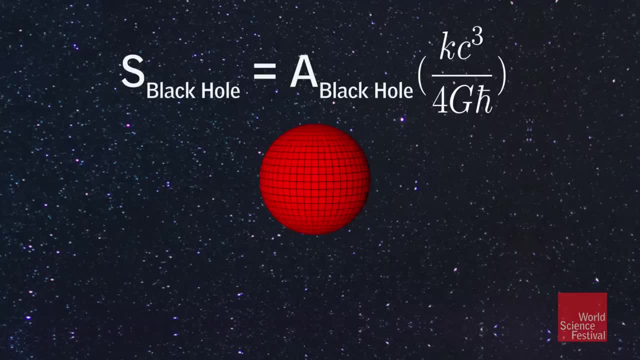 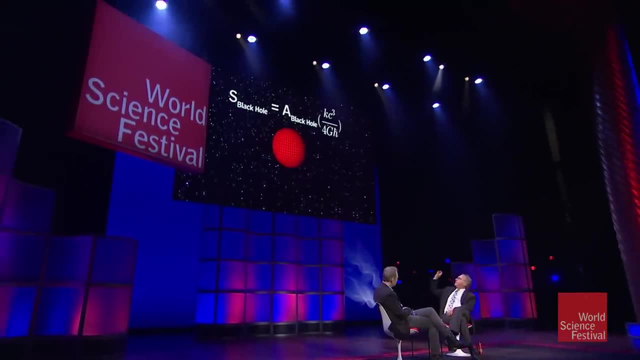 is proportional to the area, with some proportionality constant If each individual element of the information is like one square there. we just divided this sphere into these areas, So these represent bits of information on that surface of that black hole. So those little squares can, roughly speaking, 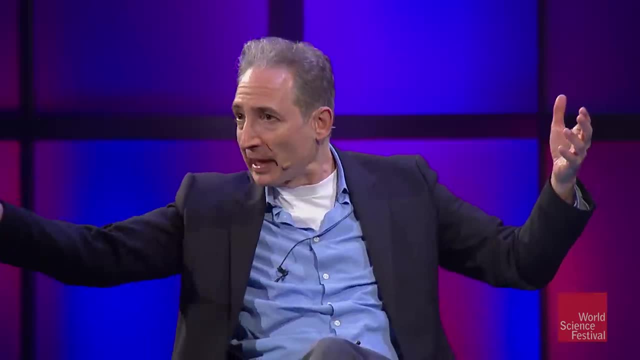 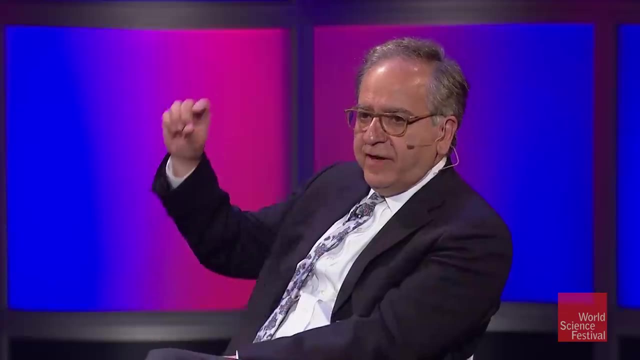 be thought of as plank areas. Using the plank length, that describes sort of the smallest length that makes sense in a quantum theory of gravity: Squares of the size 10 to the minus 33 centimeters or so, if you want to know the size. 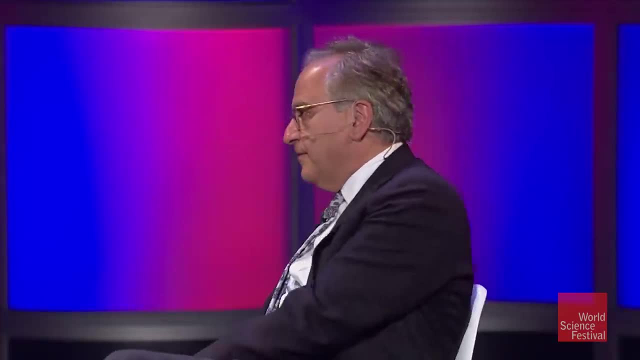 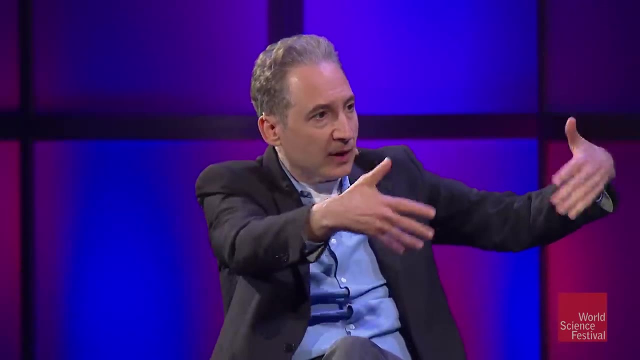 10 to the minus 33 squared Each size of the square. So you basically count the number of those little squares that are on the event horizon and that's the amount of entropy it has. So if we now took, if this is true, 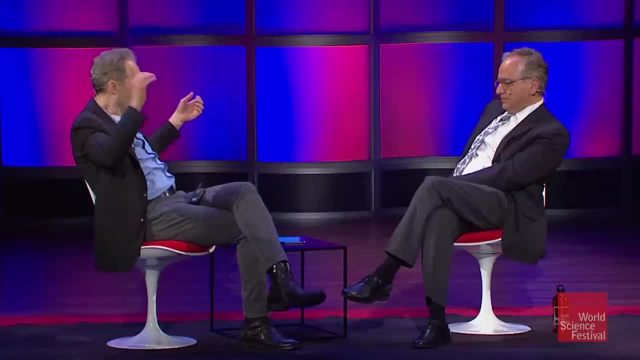 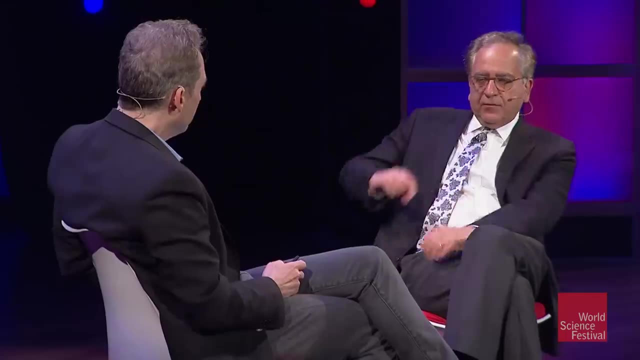 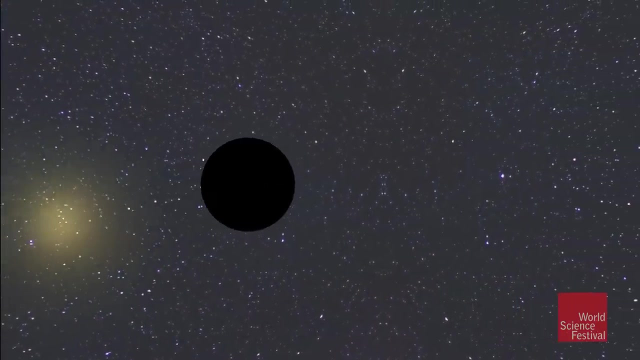 and we were to take a particle that sort of carried one unit of entropy, what would we expect to happen? if this is true, We expect this area to grow exactly by one square, So let's sort of do that We have. this is actually a real film of space here. 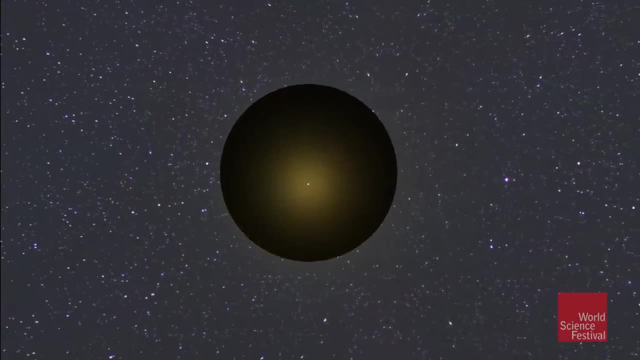 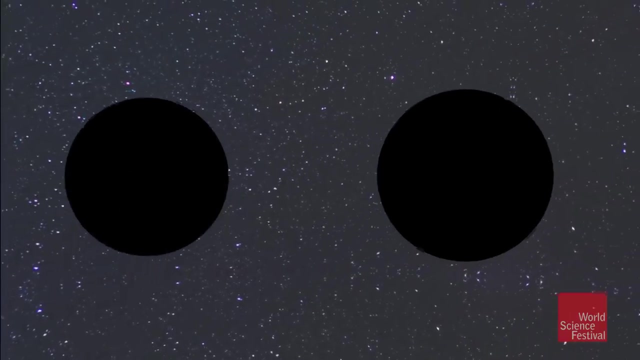 So let's get our particle going in to this guy over here. Good, So the one on the left was the original black hole. The one on the right is the larger one after a particle has fallen in. So if we take all those little squares, 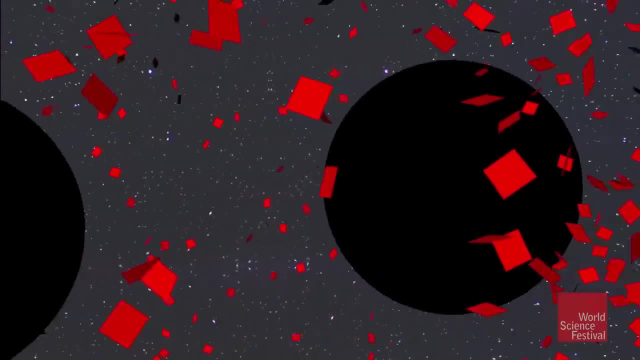 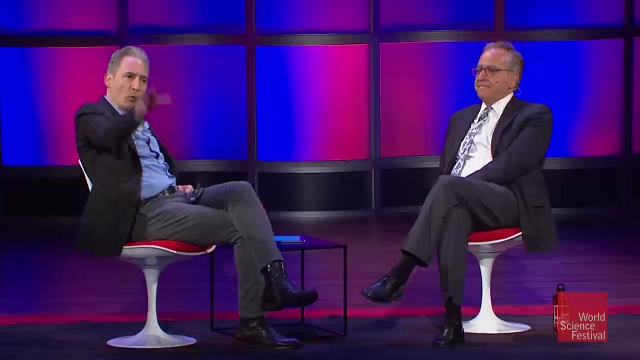 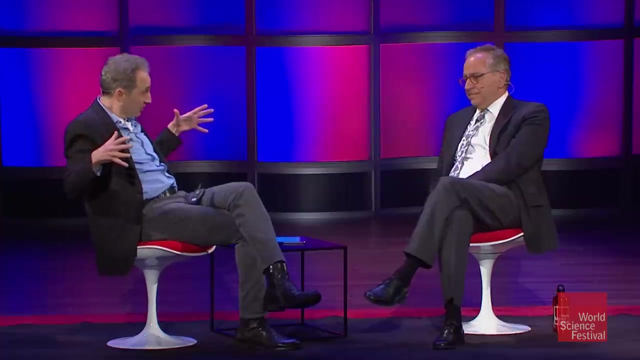 and we smear them out on the larger black hole. what we'd expect to happen is something like that, Exactly So one more square. So we throw sort of one particle in that carries one unit of disorder, and the black hole eats it. It grows a little bit. 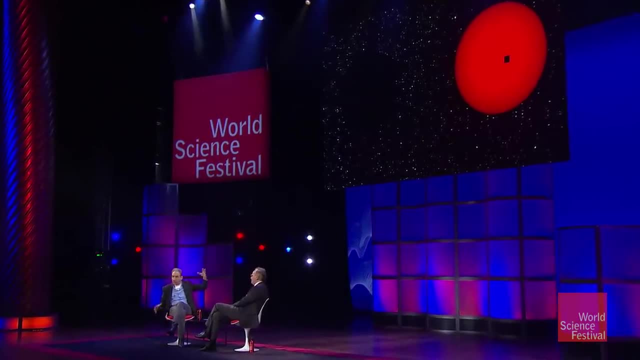 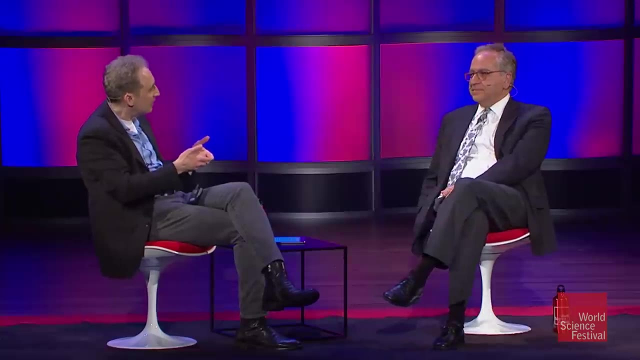 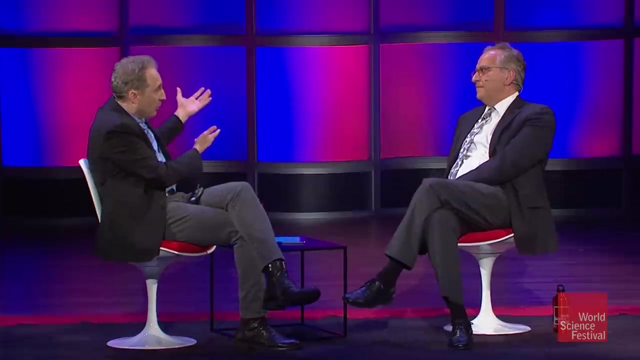 and in fact you can calculate that the amount by which it will eat and the amount by which it will expand can accommodate one more of these little tiles, and that makes this a consistent way of thinking about black holes. So this was like an important. I mean, how important was this kind of an insight? 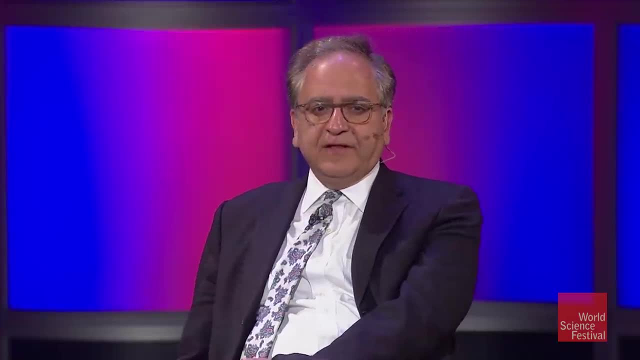 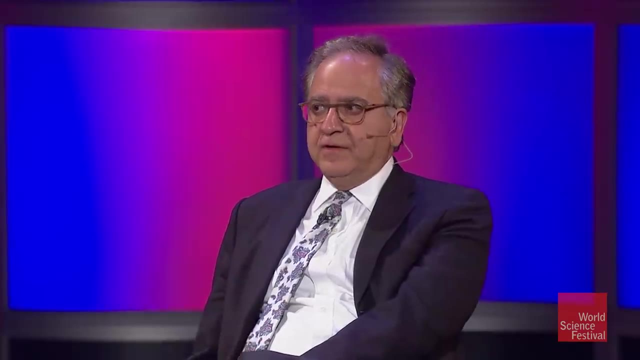 Well, it was an amazing insight, because it was the first time where Einstein's theory of relativity was combined with quantum effects, And that is what Hawking used to actually argue: that the entropy of a black hole has nothing to do with the area. And so this combination of quantum theory. 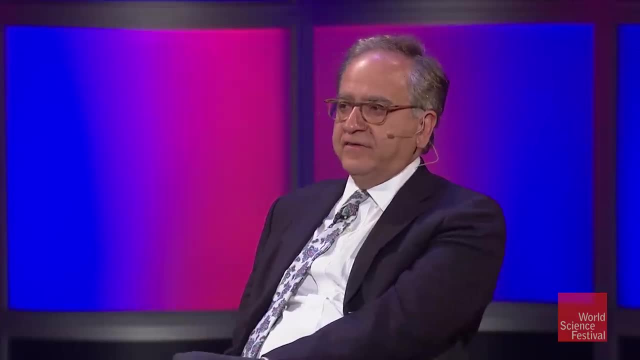 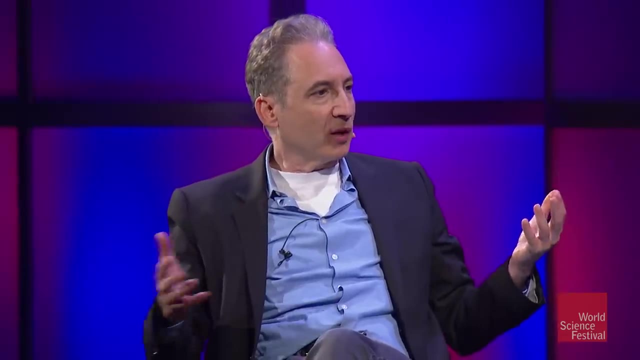 and Einstein's theory was quite novel, and this was in the early 70s- mid 70s. So is this the end of the story? when it comes to entropy and black holes Like, what issues does this leave over? Well, actually, the problem was that 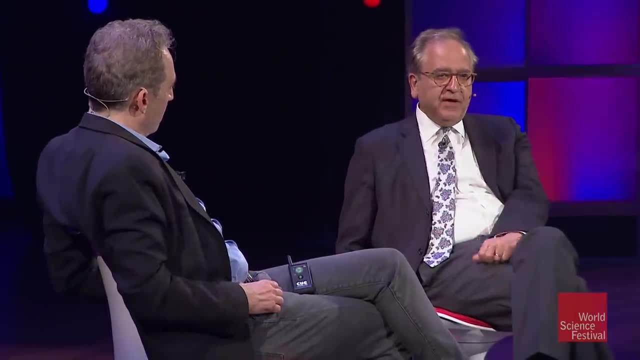 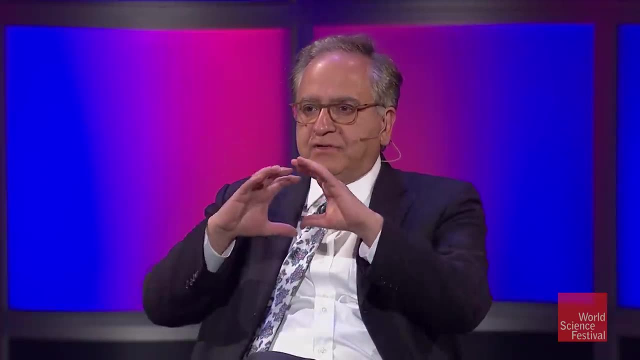 Hawking's argument showed that there must be information, but on the other hand, the horizon of a black hole is featureless, So you don't see these point squares or anything, So there seems to be no room for information to be stored on it. 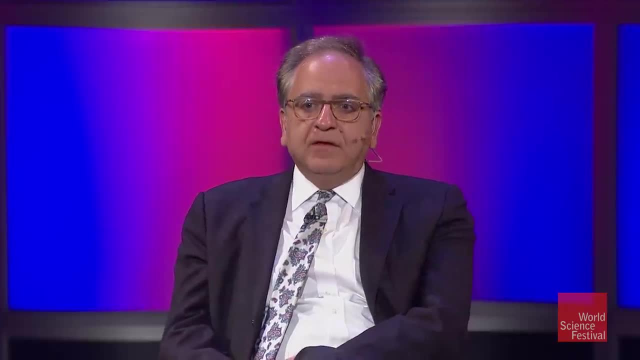 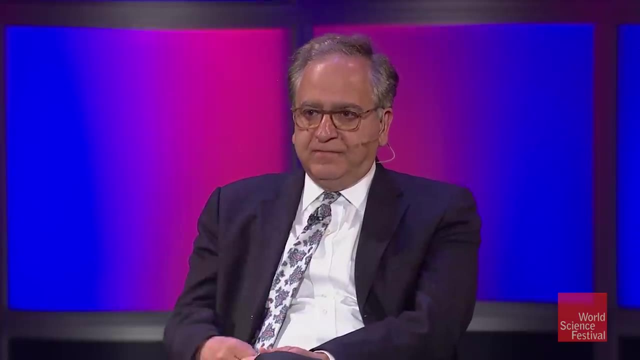 So in fact, if you use Einstein's equations and solve it, you find there's exactly one solution for a spherical, symmetric black hole. One solution means it has zero entropy. It's exactly ordered state. There's no choice. One piece of information. 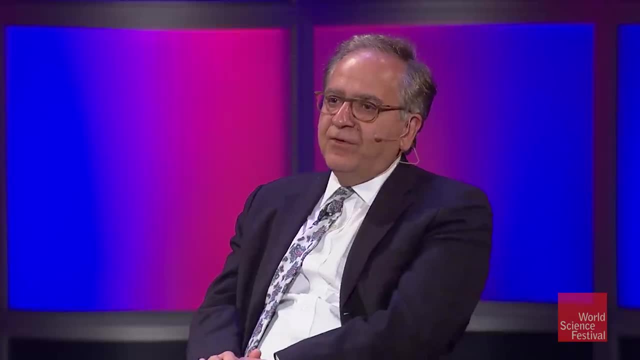 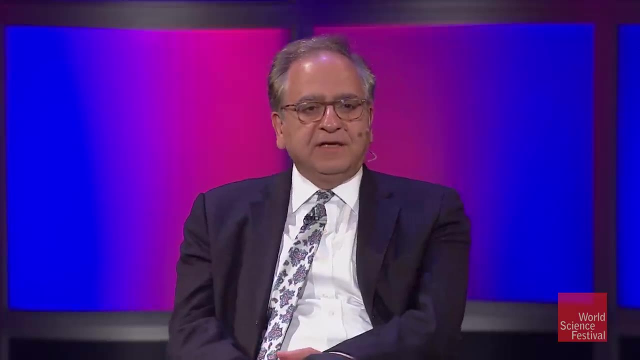 One piece of information, And that is inconsistent with what Hawking found when he combined Einstein's theory with quantum mechanics, where he found a huge amount of information. and the question is, where is this huge amount of information stored? Is it the shape of the horizon? 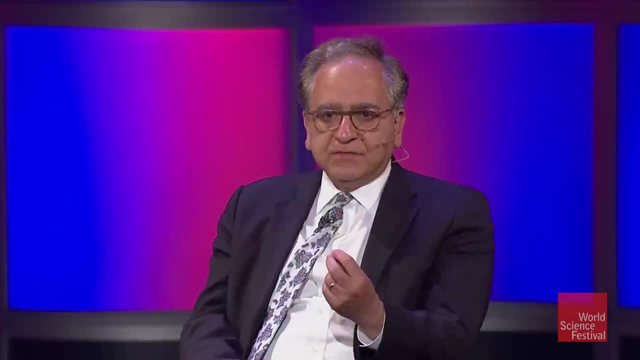 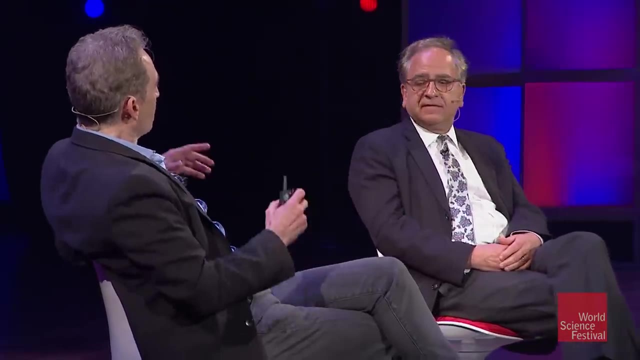 or is it what aspect of black hole encodes the microscopic structure of the black hole That was open when Hawking discovered this fact? So for Hawking's idea to work, let's just go back to my little example of sort of throwing the wallet in. 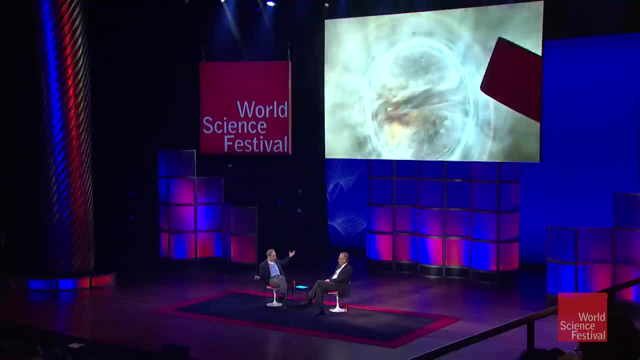 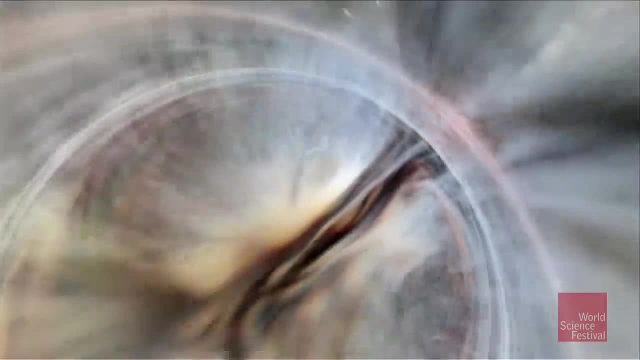 So in that little example, I threw the wallet in and said: where did the information go? So the new idea, if it's true, would be: I take my wallet and I throw it in and rather than it like disappearing, the idea, roughly speaking, would be: 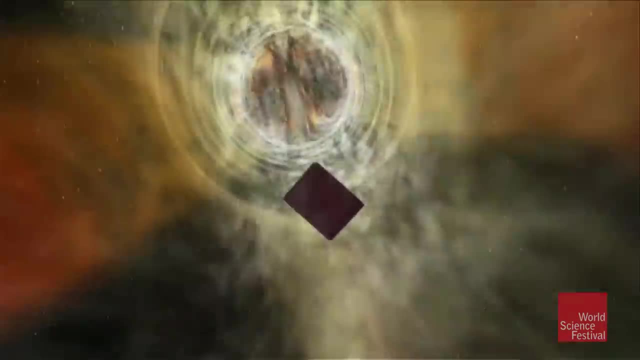 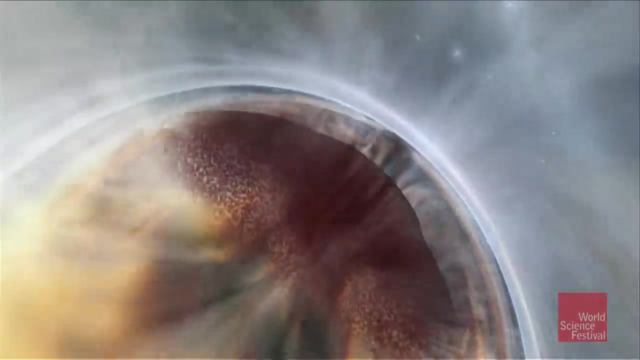 the information that is in my wallet, the configuration of all the atoms and molecules that goes toward the black hole, and we want it to be the case. that information, kind of like, smears itself out on the outside and is encoded in sort of bits, ones and zeros. 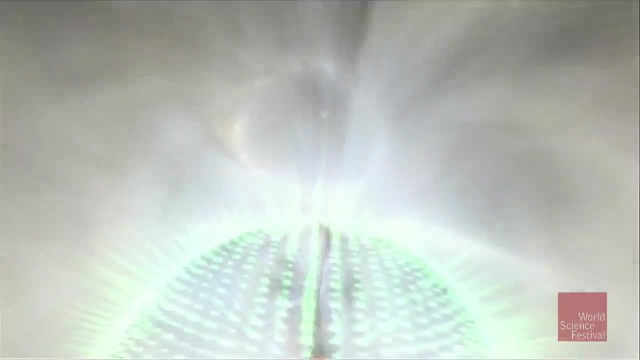 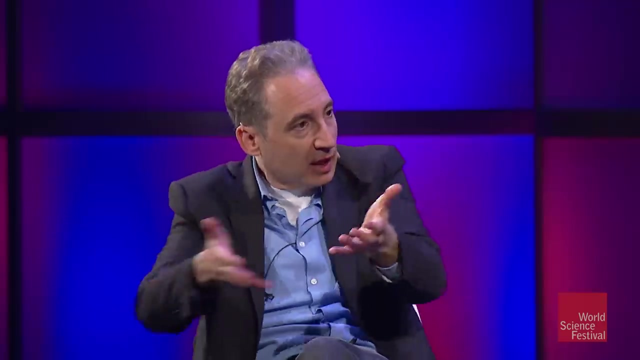 That's the picture. That's the picture And in principle, were this true, I could actually extract that information in principle and use it to rebuild anything that fell in. In this case it would be my wallet. So that's the idea, That's if the information is not lost. 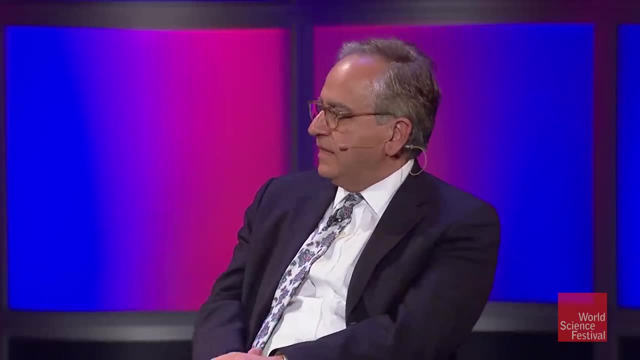 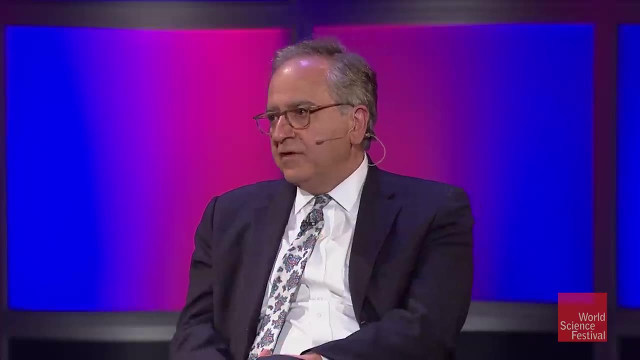 and information is there. that's what we would expect. Right, That's the hope, And the puzzle is: is that actually, Is that actually true? and how do you actually see this information, or where is it stored? or how do you account for the microstates? 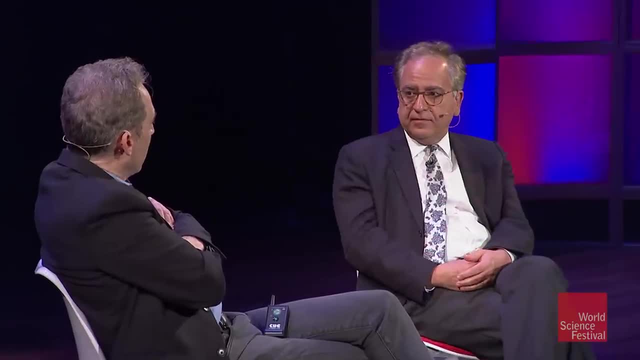 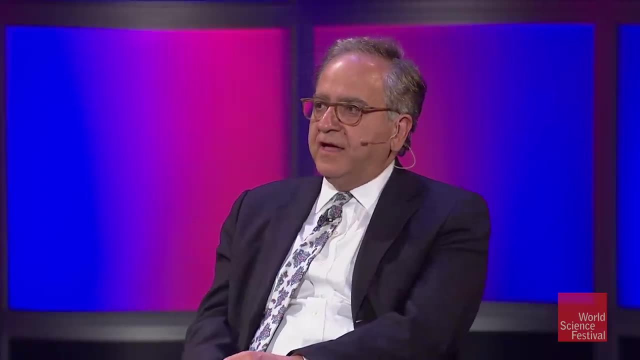 of the black hole, or the entropy of the black hole, And that's where you come in. Well, me and my colleagues in string theory began studying these questions more seriously with the advent of duality symmetries in string theory. So first, perhaps I should say: 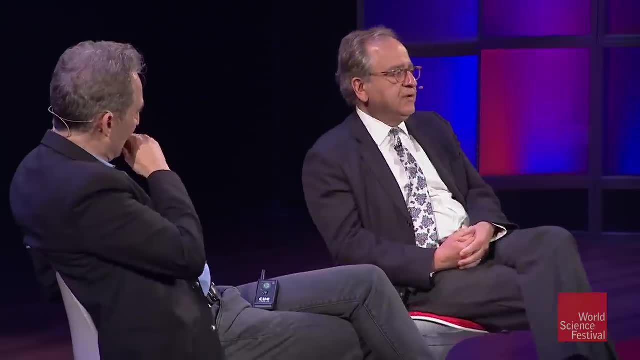 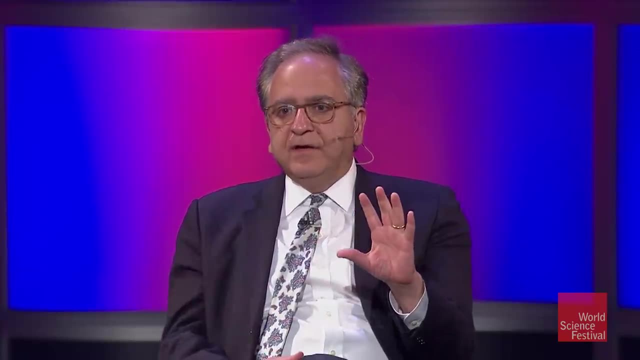 So first, string theory. Can you say a few words about string theory? I should say a few words about string theory. So string theory is a framework where we believe combines Einstein's theory of relativity with quantum theory in a consistent framework And as part of it. 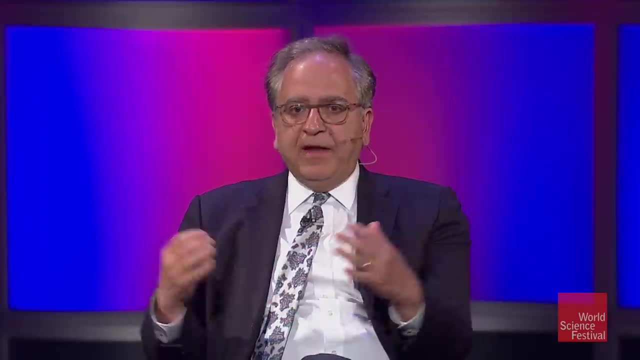 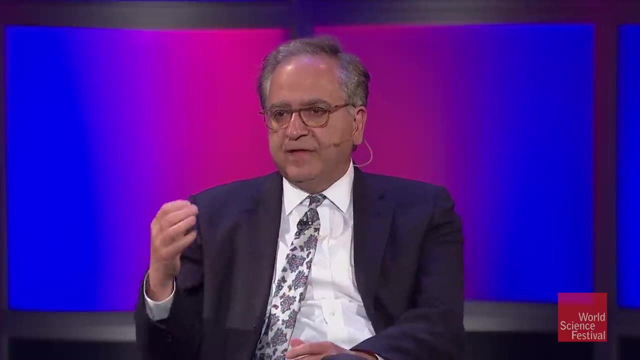 it demands that the entities making up the matter are not just point particles, but entities like strings or membranes or extended objects have to play a key role. So that's one aspect of string theory. So here's a little if you want to take us through. 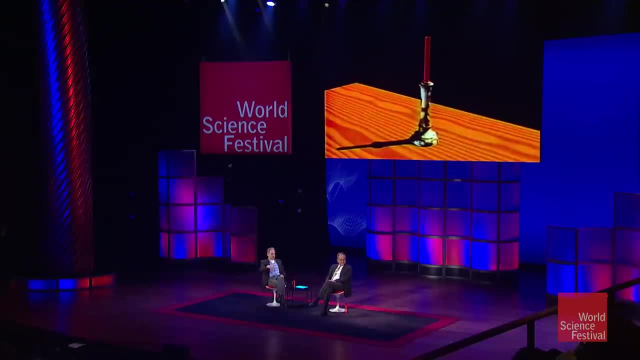 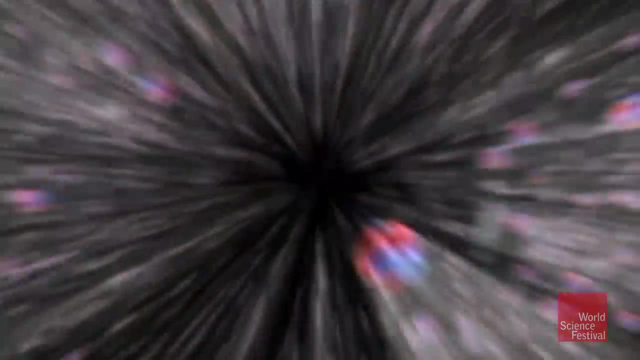 this is just a little example of what string theory might look like. So you got a piece of matter and we're going to dive into it. and then you're saying that if we go sufficiently deep, So if you go to the beginning inside, you'll see the atoms first. 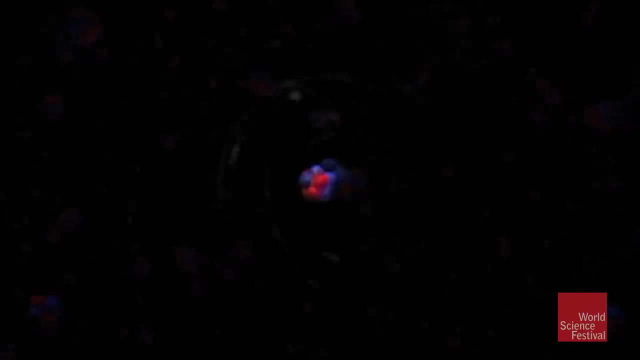 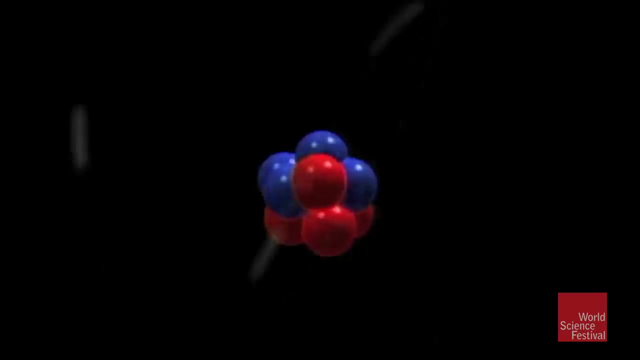 and you know, inside the atoms you see the nucleus, and the nucleus you see- well, here I guess the protons and neutrons, I'm assuming, and you go inside them, you see the quarks. and once you see the quarks, you can go inside them. and if you zoom in a little further, 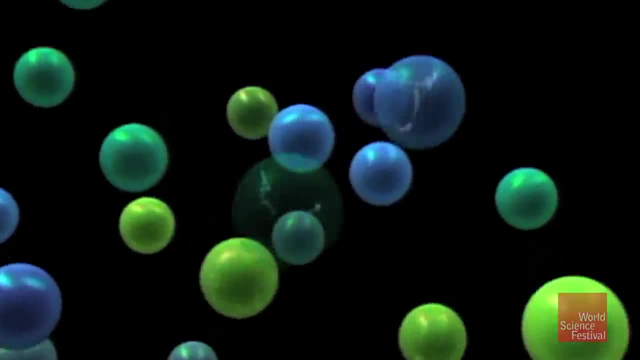 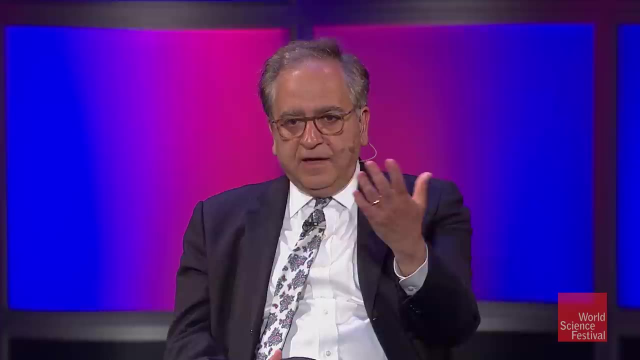 you might see, actually, that these featureless quarks that you think are point particle actually are tiny strings, vibrating strings of some sort, and that's the kind of a picture that we expect to be true in the context of string theory that point particles are point-like. because we are not zoomed in sufficiently close to them, and if you zoom in enough, they will have features like strings. How big would those? We don't know exactly, but it could be like 10 to the minus 30 centimeters, somewhat close to the Planck scale. 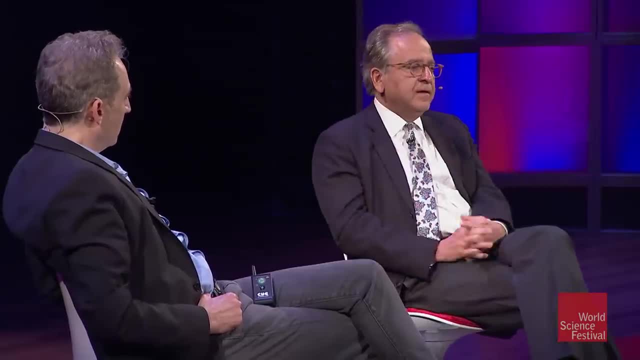 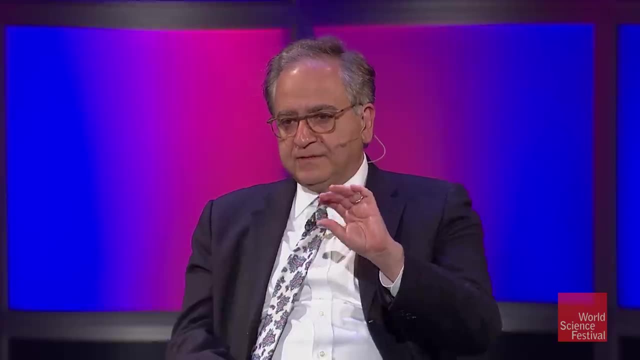 that we discussed already in the context of the areas of the horizon of the black hole. So that's the basic feature of string theory. but as one of the aspects of string theory that was originally one of the negative features was that string theory predicted that the spatial dimension of the universe 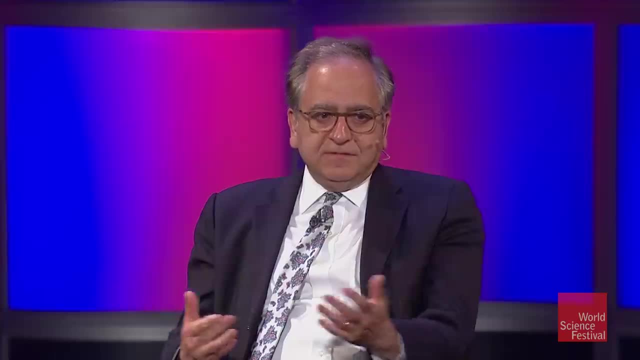 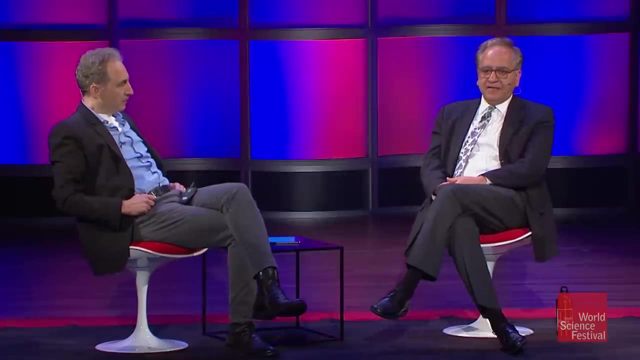 is not three, and that was manifest in contradiction with the fact that we think we live in three spatial dimensions. we have three spatial dimensions. string theory seemed to demand that we have nine spatial dimensions, and so this was a contradiction originally, and physicists thought: how could this possibly work? 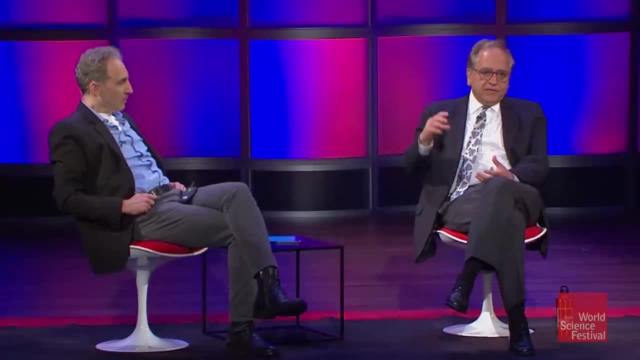 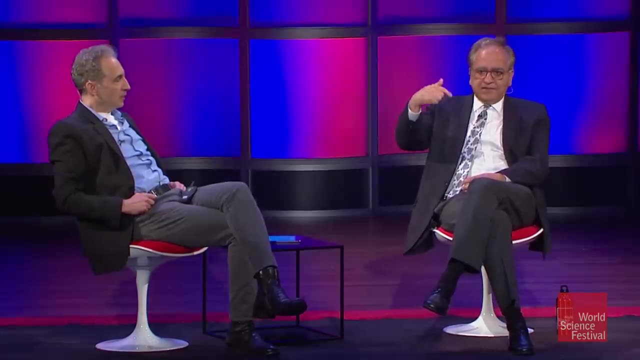 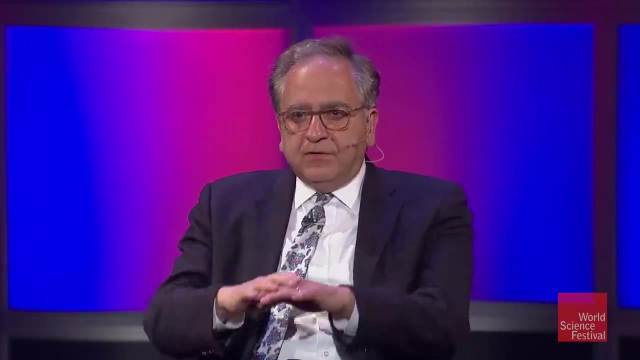 and one resolution was: oh, these six extra dimensions that we have are so tiny, like little circles at every point in space. let's imagine six circles at each point, six types of circles which are so tiny that you cannot see. so the idea would be the macroscopic dimensions. 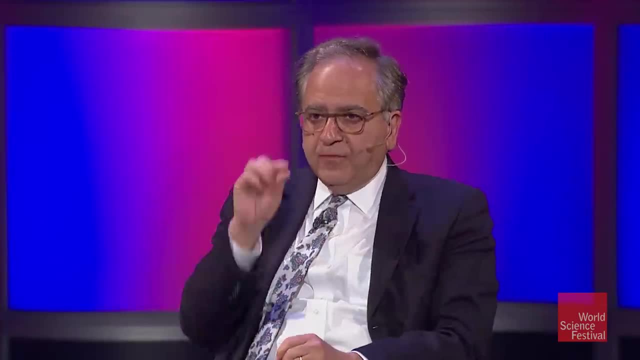 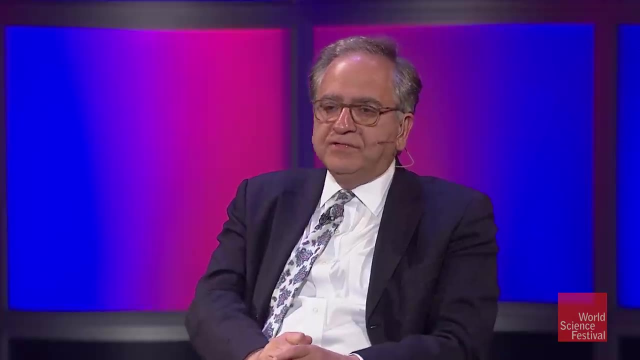 are only three. the big ones are three but the tiny ones are six. and the tiny ones are hard to see unless you really zoom in. and that's difficult to do with the energies that's available to us in our experiments today, But the idea would be. 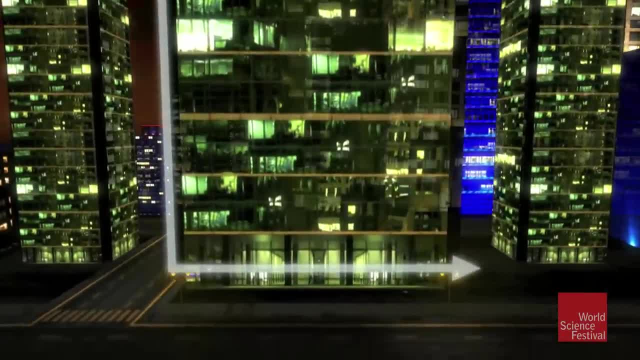 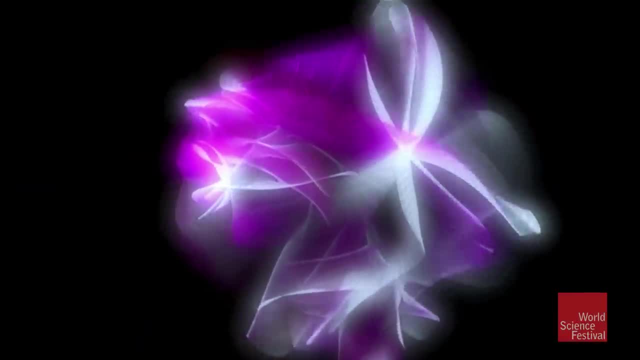 that you've got these big dimensions, that we know about these extra dimensions, and then how do you relate this to this idea of black holes? So this was actually a negative feature for string theory, so string theorists were kind of struggling. yeah, we have these six extra dimensions. 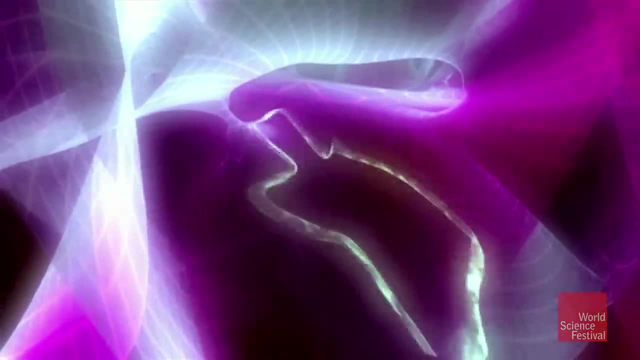 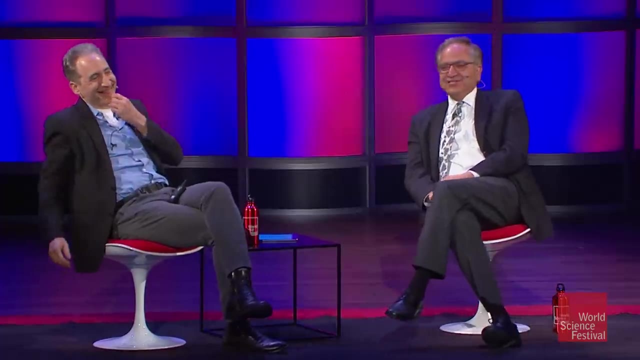 it's a little embarrassing, it's tiny, you don't see them. and then other people said, sure, sure, yes, yes. so this was the state of the art till mid 90s, where we didn't know what to do with these extra dimensions. they were there. 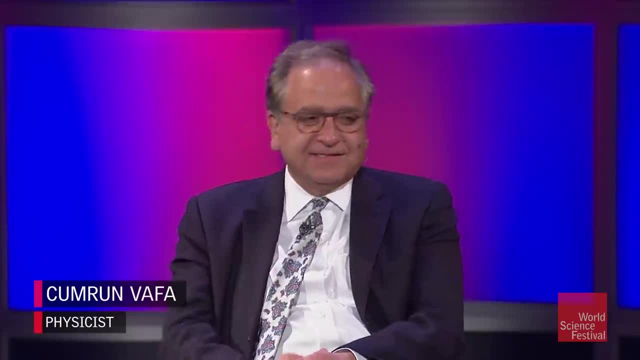 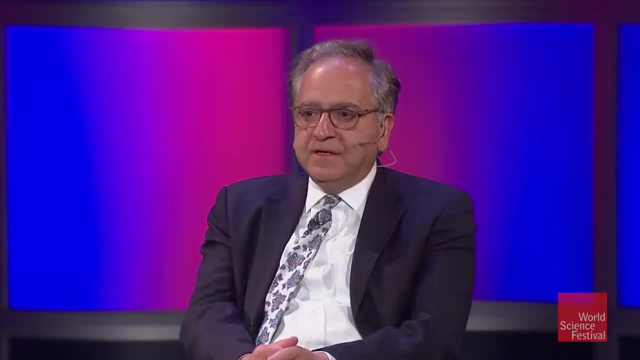 just to make the theory consistent, and we were hiding it away in tiny little things. and then came the question about the black holes, and the black hole had the opposite problem. the problem with the black hole was we were missing information of the black holes. where were they? 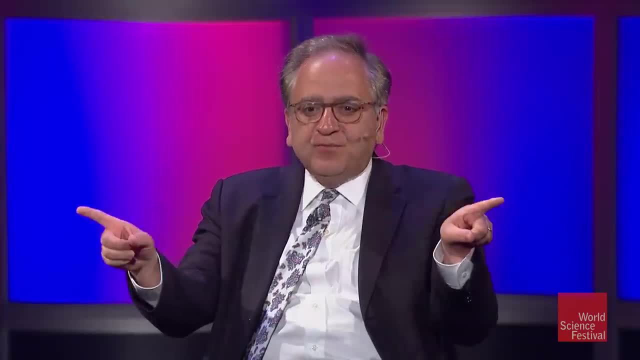 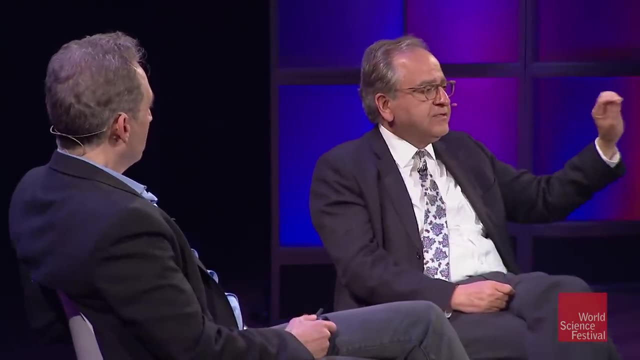 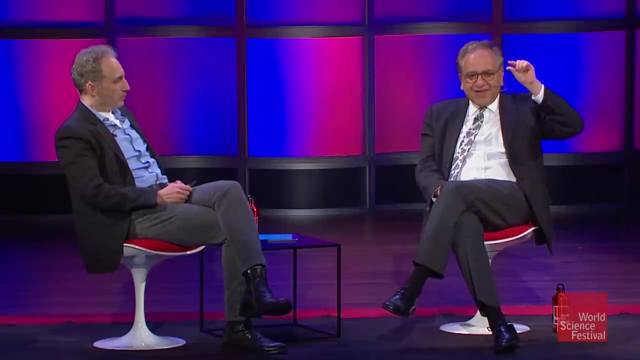 what were that information? it turned out that these two problems cancelled each other out, and so the problem that was, where are the ingredients or the degrees of freedom that constitutes black hole, ended up in the internal spatial, tiny spatial things that I was talking about. so, as you can see here, 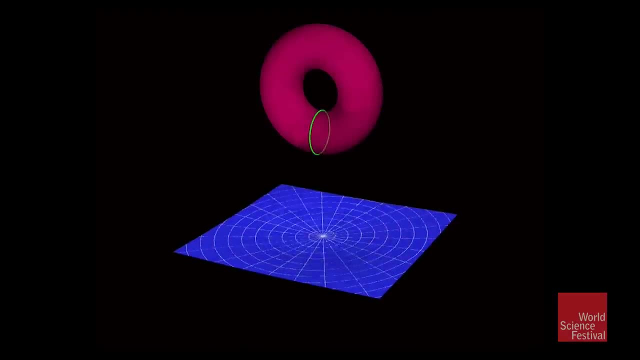 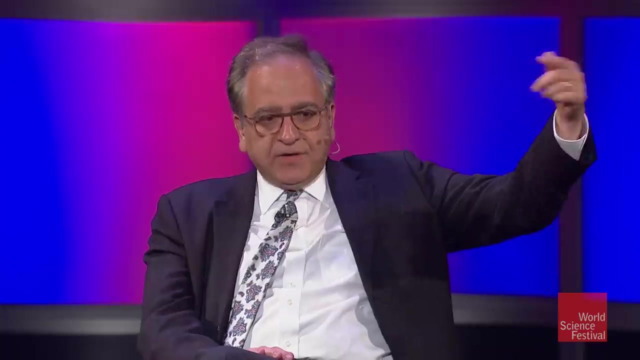 the red donut shaped object there is to represent these tiny internal dimensions, and the blue sheet that you see represents the macroscopic, three macroscopic dimensions, and so the idea there is that if you take a string or a membrane or one of these extended objects and wrap it around the cycles, on these external tiny spaces, like a torus or like a circle or a donut or what not shape you have. it will create a mass at the point where you are wrapping around that circle and the more it wraps around, the more mass is going to be constituting it. 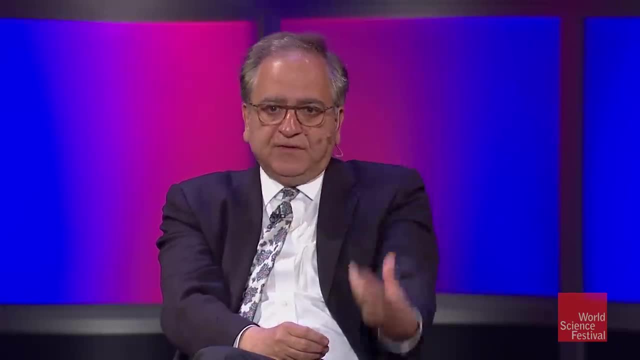 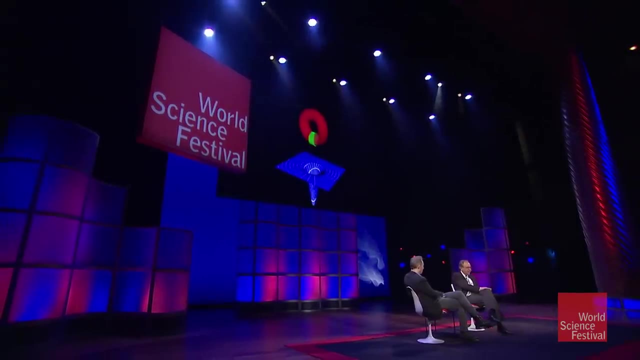 and the more it's going to shape and distort the geometry of space around it and if it's enough of it, it's going to create this warped space which is what we call the black hole. so the black hole itself can be viewed as these strings or membranes. 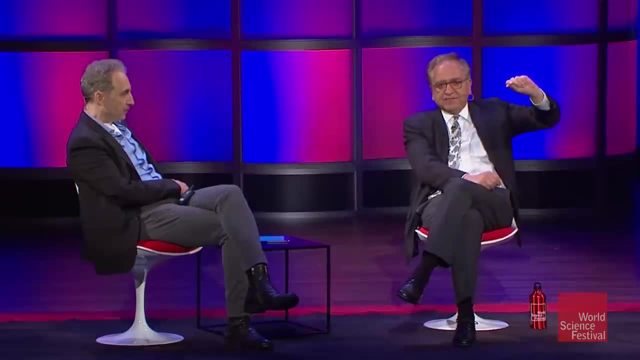 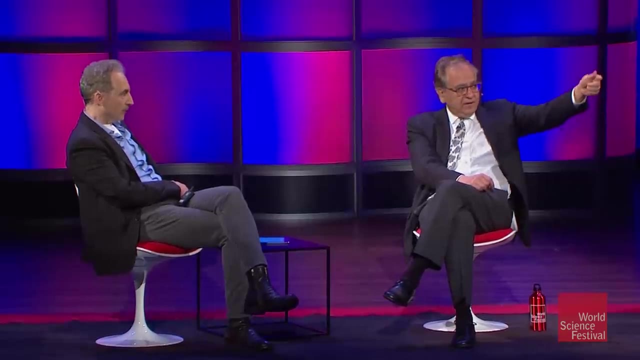 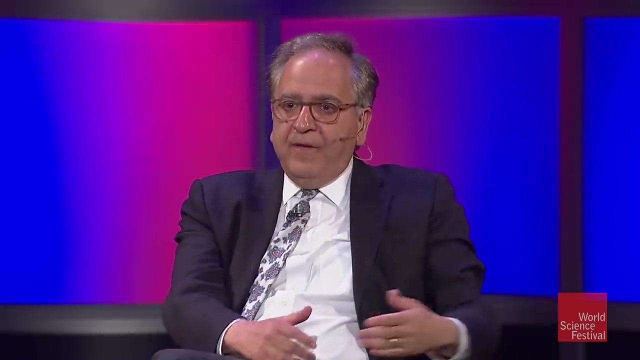 wrapped around these extra cycles of this tiny space. and so then, if the question is: what accounts for the degrees of freedom of the black hole? these are precisely these strings or membranes wrapped around these extra dimensions. how many are there? how many degrees of freedom are there? what are the entropy? 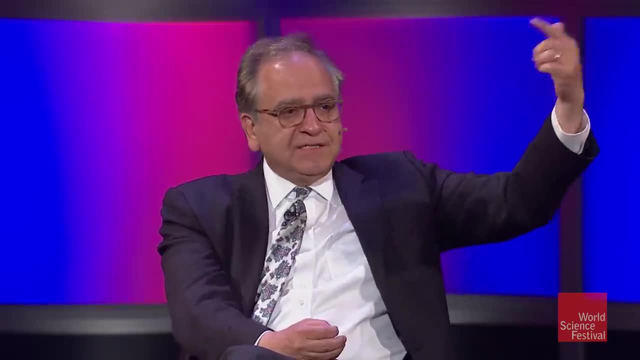 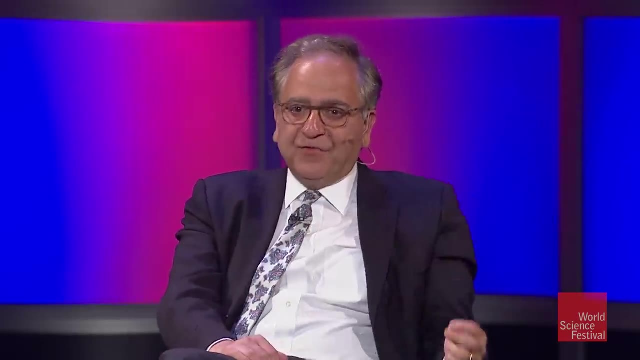 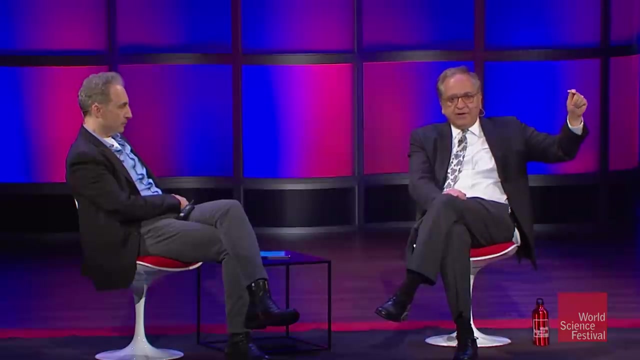 gets translated to how many ways these extra strings or membranes can wrap around these extra dimensions. and there are many ways and that accounted for the entropy of the black hole. so with Andy Strominger and I did actually a computation of how much entropy is there in these wrappings of these strings. 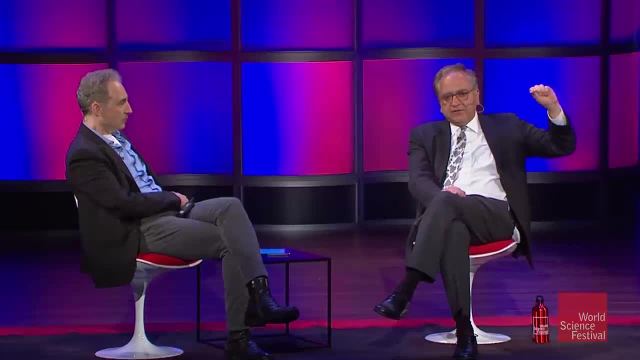 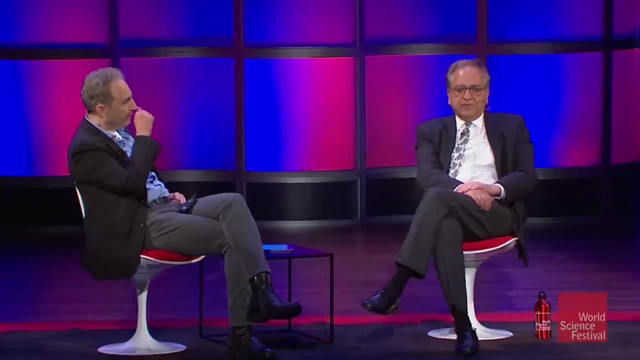 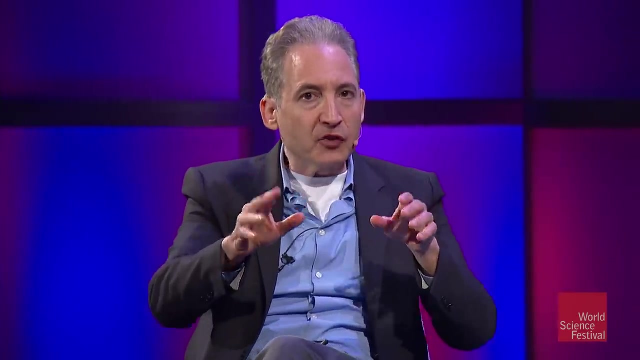 around the external, around these internal dimensions in string theory, and we found exact match with the prediction that Bekenstein and Hawking had made about the entropy of these black holes. so just to quickly unpack a little bit: so basically, you found a new way of describing black holes in string theory. 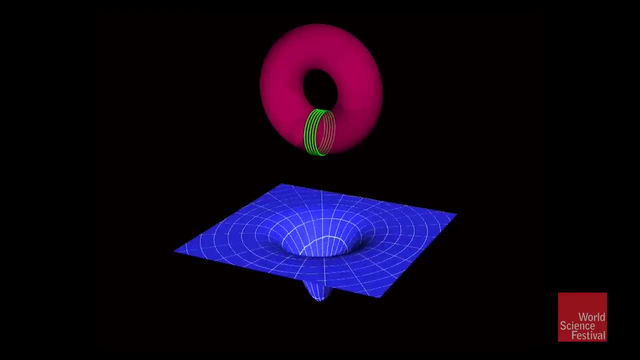 which makes use of the extra curled up dimensions, the red part of this image that we find here. and you're saying that by wrapping these strings or ingredients of string theory around the extra dimensions, you can create a warping in space that looks just like the black hole. 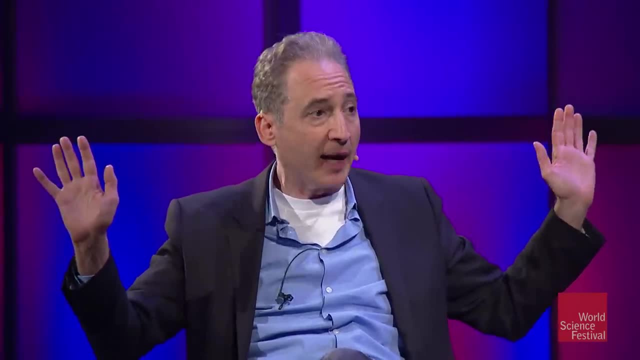 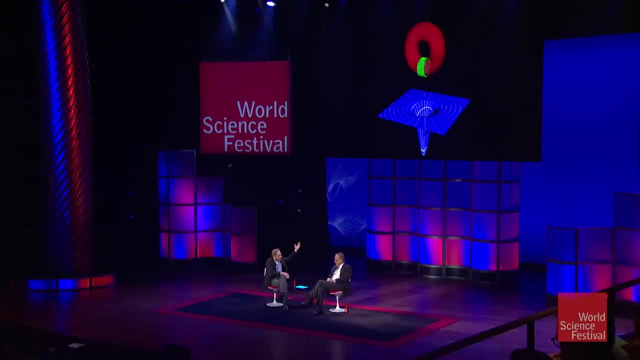 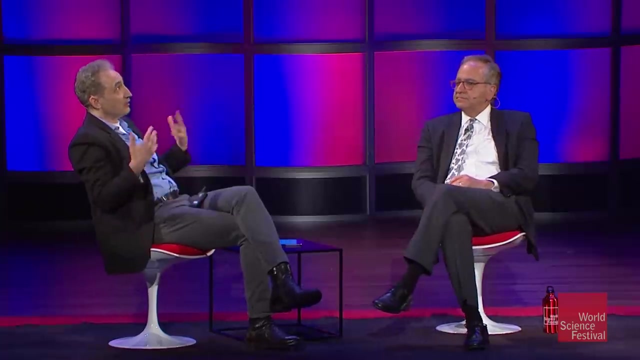 that we've been talking about for many years, before string theory even was on anybody's mind. but in this description you can do a direct count of the amount of information necessary to describe the situation and, bang on, it matches what Hawking said, so this gives us insight. 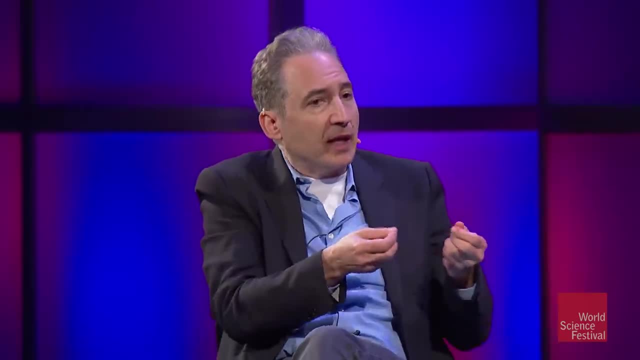 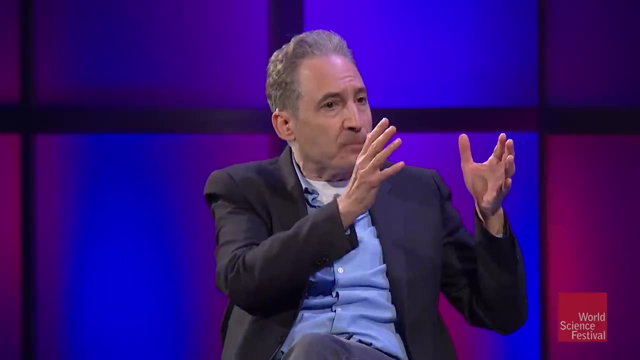 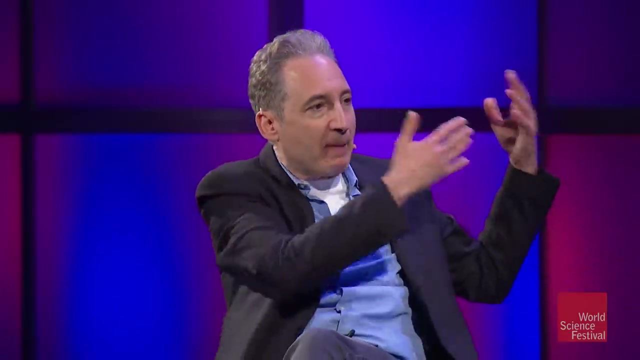 into one possible way of describing the internal structure of a black hole, which in many ways I think the community views is one of the most important pieces of data that string theory may be going in the right direction. we don't have experimental support for these ideas, but here's a mathematical piece. 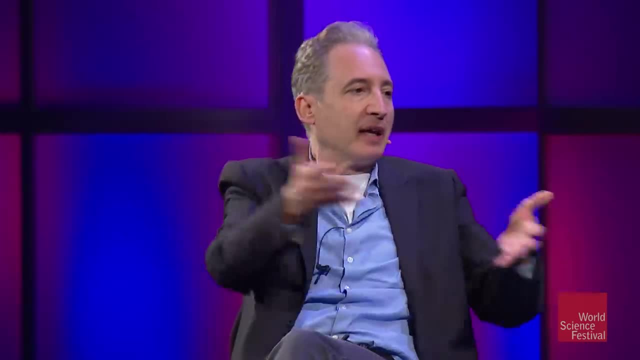 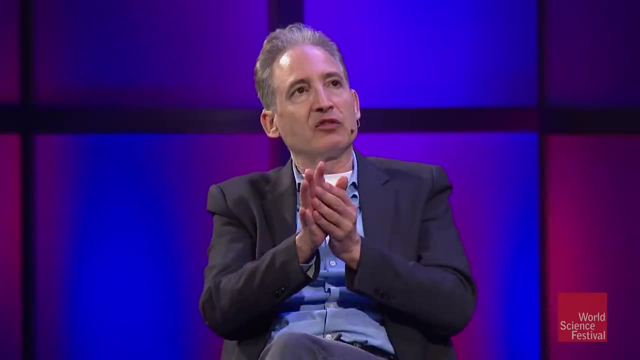 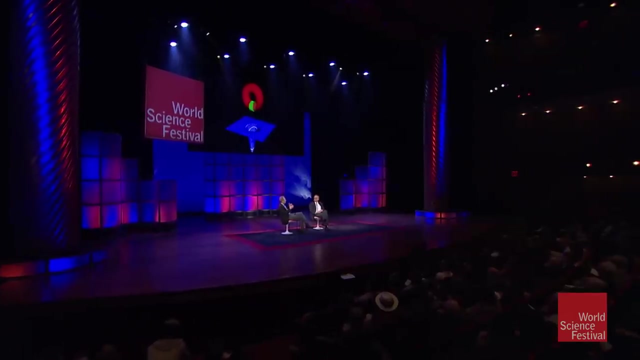 of experimental support, if you will- that it matches ideas that have been on the table for 25, 30 years. so this isn't a key step forward. but now let's turn to some of the puzzles that still remain, and part of the puzzles surround something. 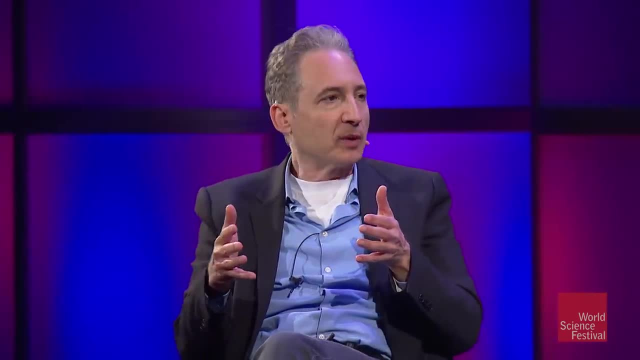 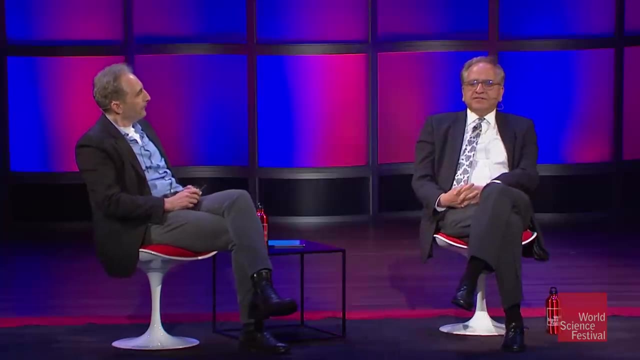 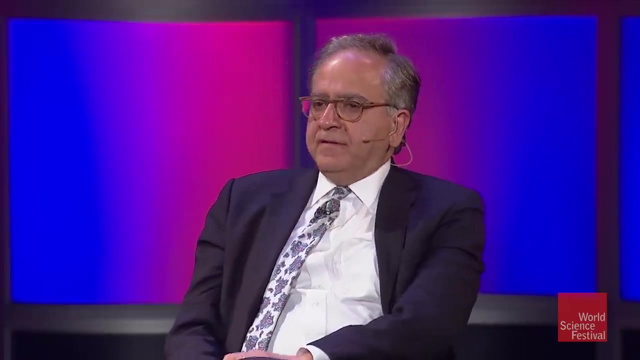 that's tightly related to what we've been talking about, which is something called Hawking radiation. can you just tell us a bit about what Hawking radiation is? yes, so Hawking. after discovering the properties of having information in the black hole and the entropy, he also noticed that the black holes 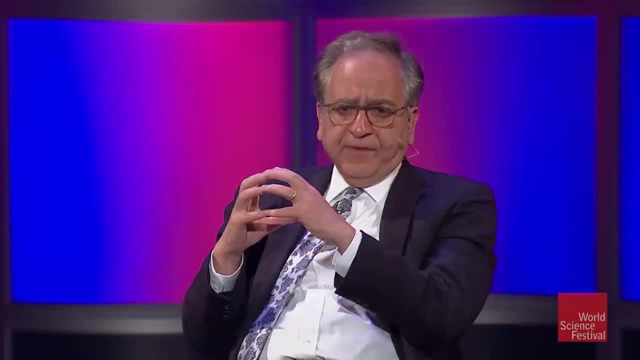 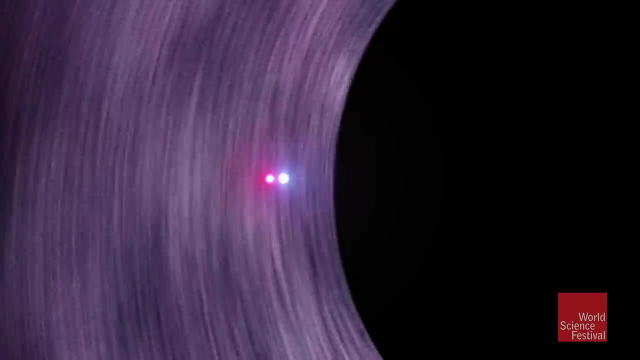 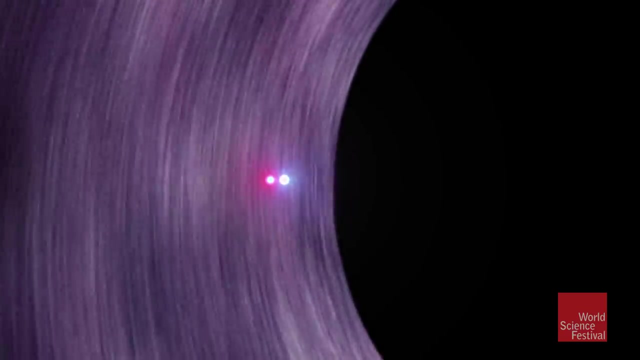 actually are not quite black. and what happens if you go near the event horizon of the black hole? what happens is that you get pairs of particles created out of vacuum. these are quantum fluctuations. the quantum fluctuations are always creating particles and anti-particles in pairs and typically they go in and out. 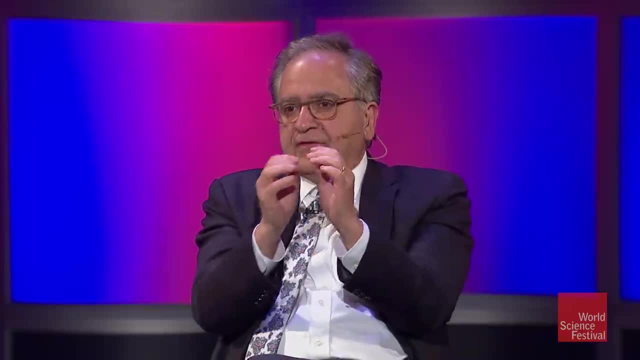 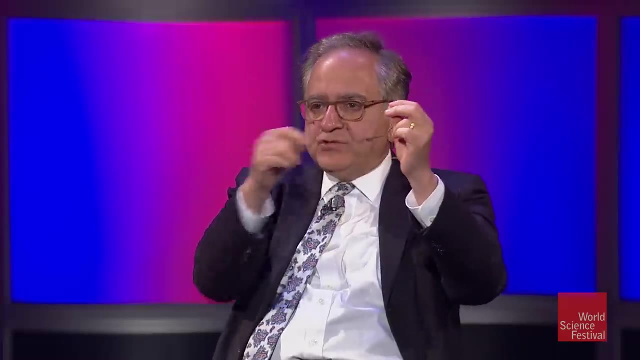 without doing anything. but if they are near the event horizon, one of them, per chance, could go towards the inside of the black hole, and then one of them could go outside, and the one which goes inside has no way of getting out, so it's stuck there. but the one going out 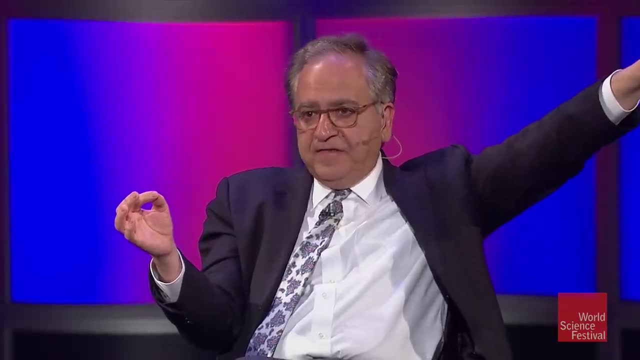 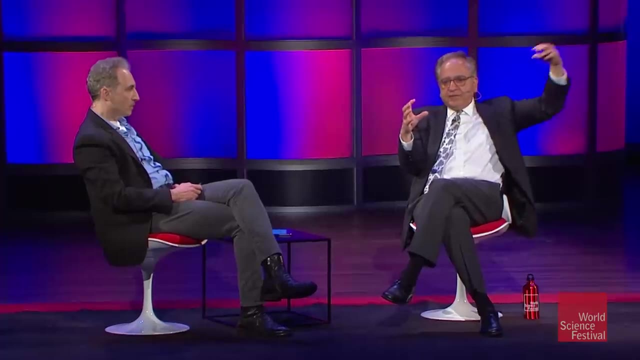 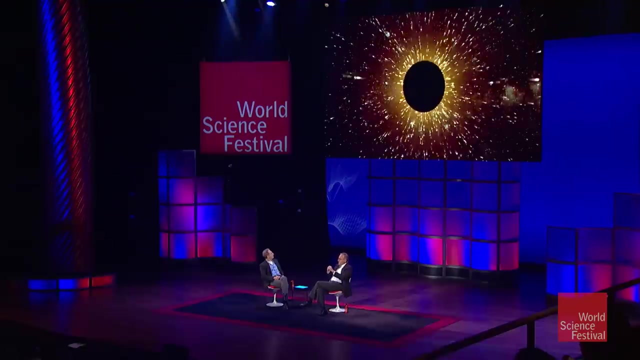 can leave and go far away from it, all the way to infinity, and that looks like a radiation from the viewpoint of somebody outside. so, in other words, from the viewpoint of somebody outside, the black hole is actually radiating energy. as it radiates energy, it loses mass. 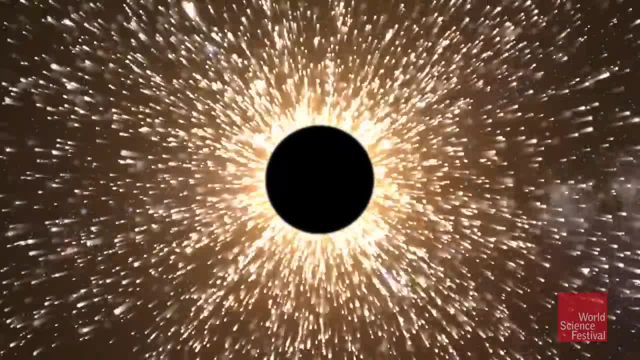 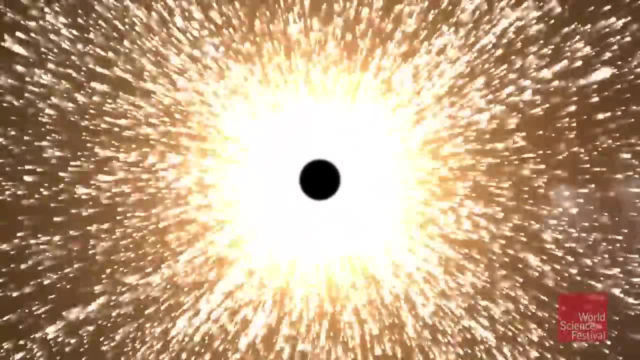 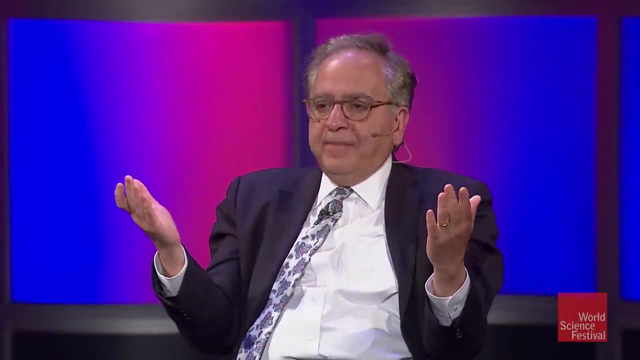 and it shrinks and shrinks and shrinks until after a while, the black hole totally disappears, where there is no more energy left to emit. so once the black hole disappears, the question is: what happens to all that information that went into the black hole? what happened to that area? 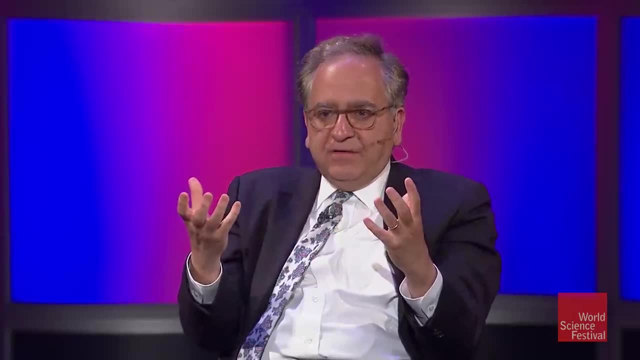 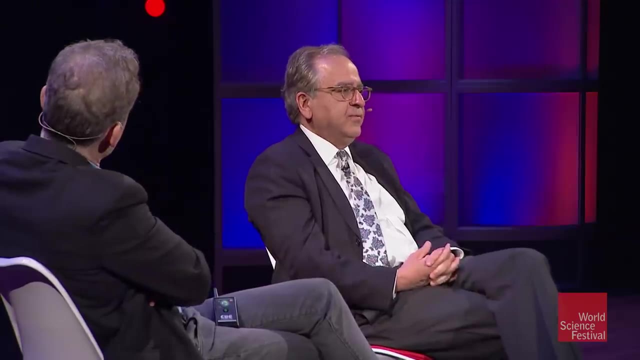 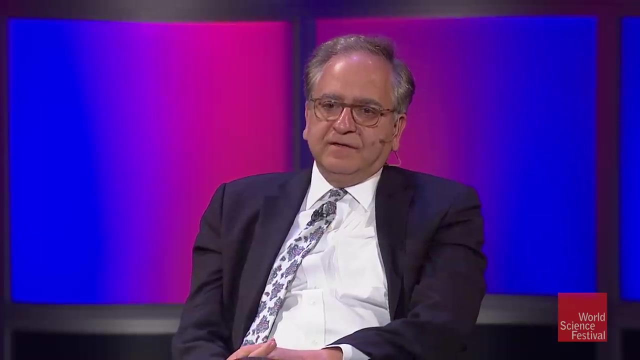 I was talking about. where is that information gone? so this was a question that Hawking basically posed. perhaps you recall the discussion between Einstein and Bohr that Einstein did not like the probabilistic aspect of quantum mechanics, and so he said: God does not play dice, and Niels Bohr responded: 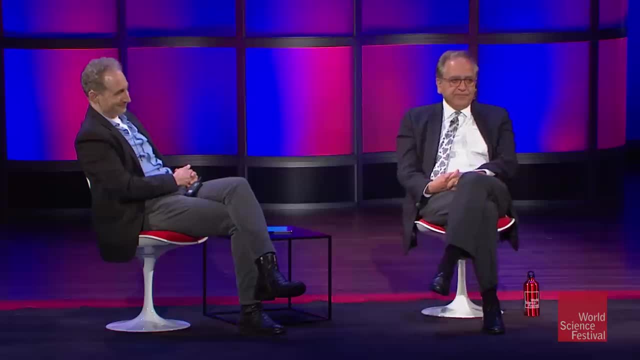 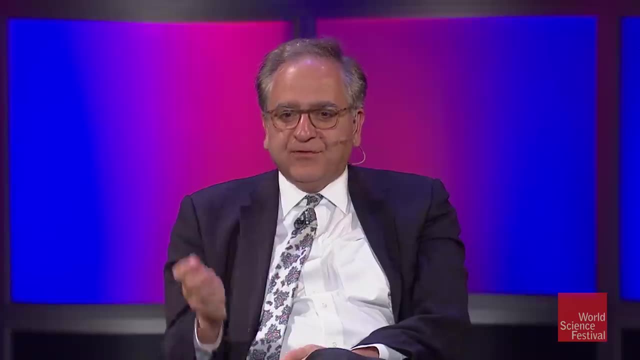 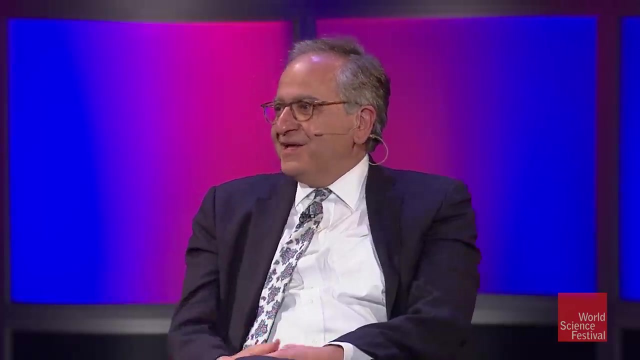 by saying to Einstein: stop telling God what to do. and Hawking added his own wrinkle on this and he said: well, what happens if you throw a dice inside the black hole? and the black hole after a while disappears, and with it disappears the dice. so, and then he said: 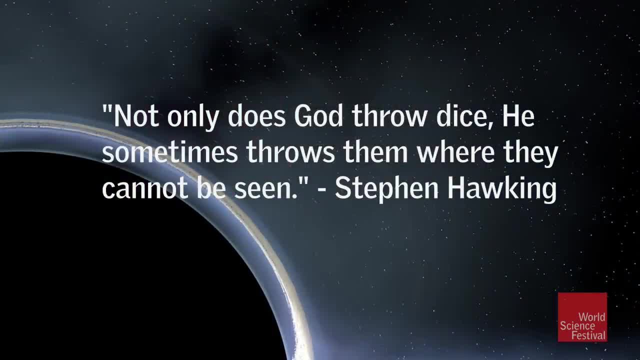 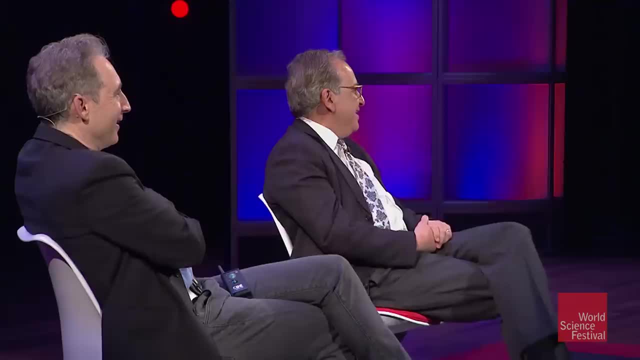 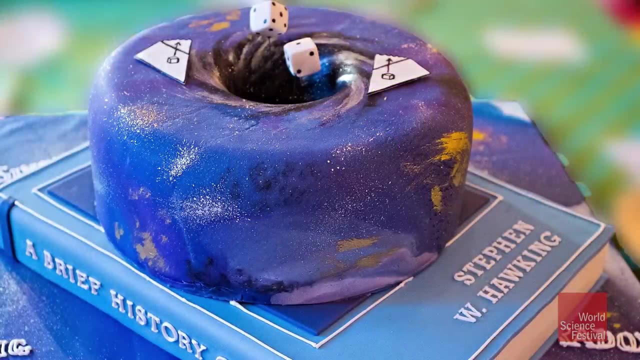 not only does God throw dice, he sometimes throws them where they cannot be seen. and then you made a little cake. so, yeah, we had the lucky occasion of having Stephen Hawking as our guest at our home a couple of years ago, when he was visiting Harvard, and we made a cake. 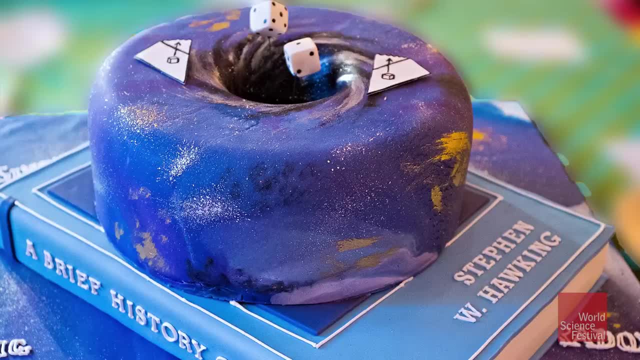 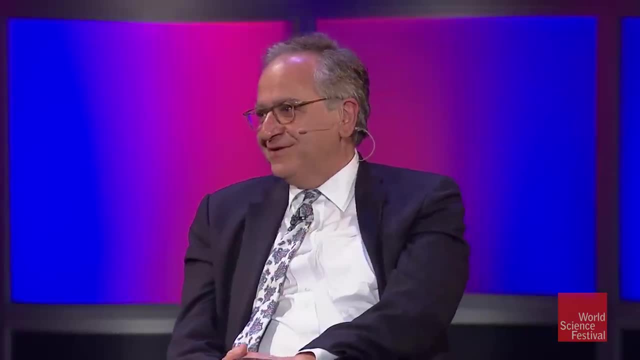 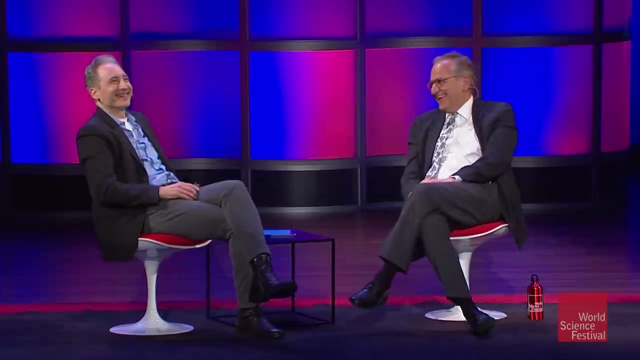 in the form of a black hole with the dice and the book. his famous book, which is actually made of, is a cake and it's actually gluten free because he was allergic. so Stephen had his cake and he could eat it too. very nice, so in that picture, 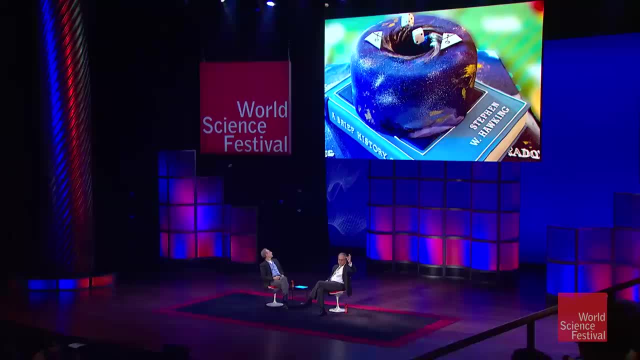 you see that there are two dice hanging there, floating towards the black hole, and it's going in, and that's the issue of the information puzzle. you lose the information of what is the dice roll, and that's what's called the information puzzle, because if the dice rolls, 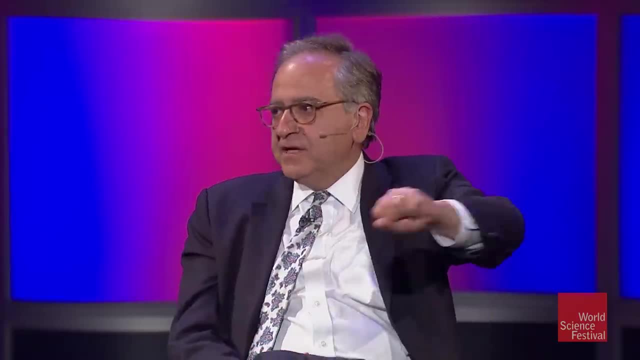 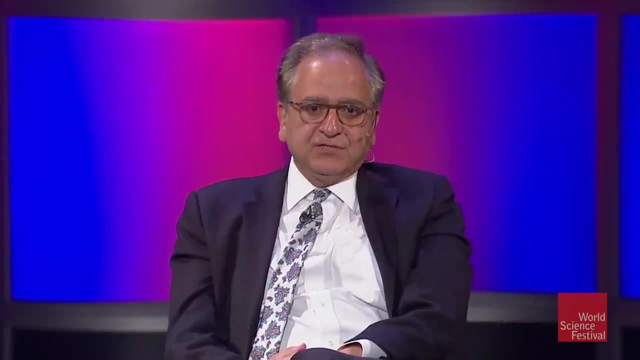 some number and the black hole evaporates and disappears. with it disappears the information about what the roll of the dice was, and that's called the information puzzle, which we still are struggling to understand even today. now, most people in the field for a long time have anticipated. 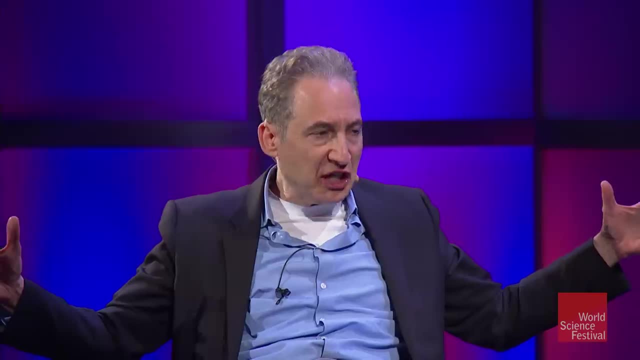 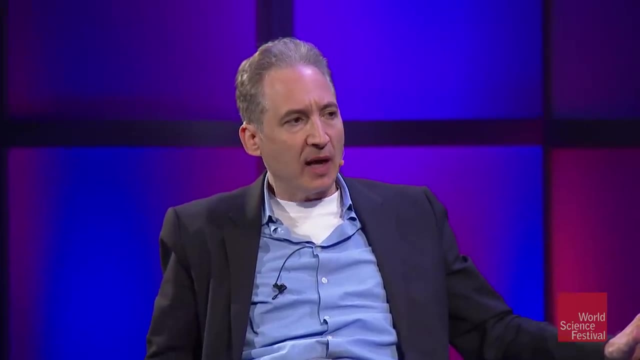 the fact that somehow the information does get out with that radiation that we saw coming off of the black hole now for a while. Stephen Hawking said that the information would not come out. I mean, that quote was quite serious. he was saying that we have to rethink. 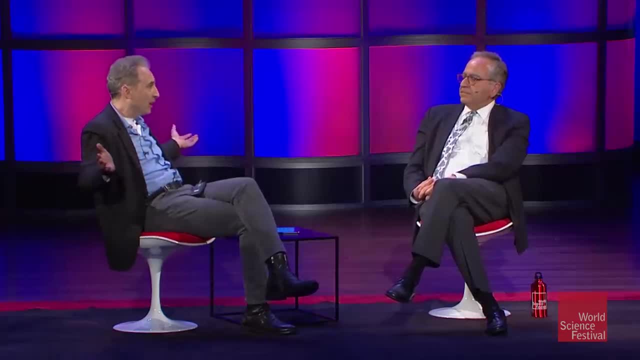 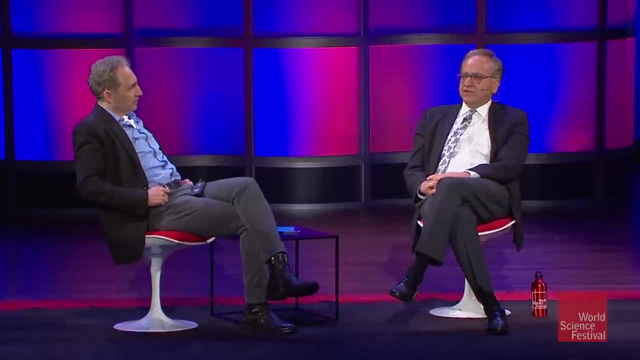 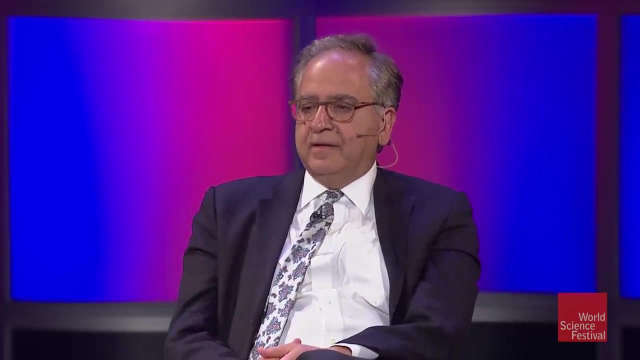 quantum mechanics, because the information does not come back out. he then changed his mind on that. yes, so part of the reason for this is the discovery of a more detailed version of what is called holography. in other words, this began with the work already back in the long time ago. 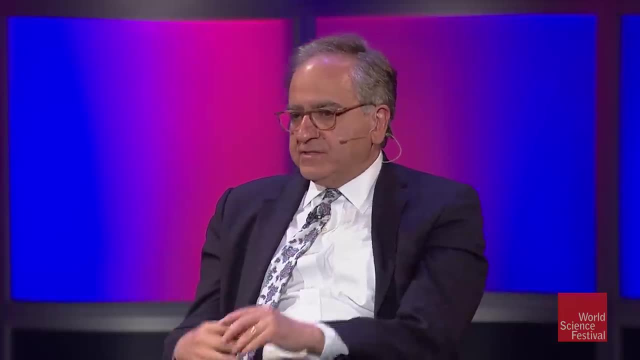 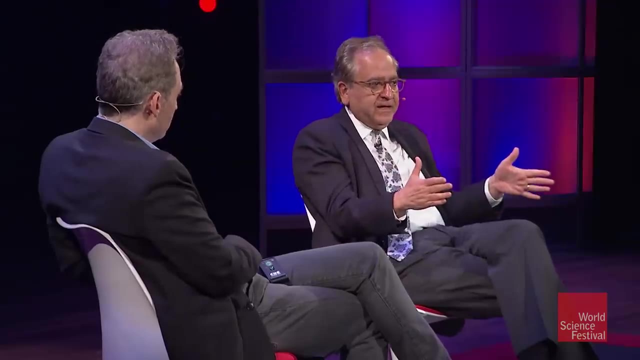 but became more precise with the work of Juan Maldacena, where it was discovered that you can describe a gravitational system precisely using objects which are much simpler to understand and, in particular, in that system you could prove mathematically rigorously. there's no way. 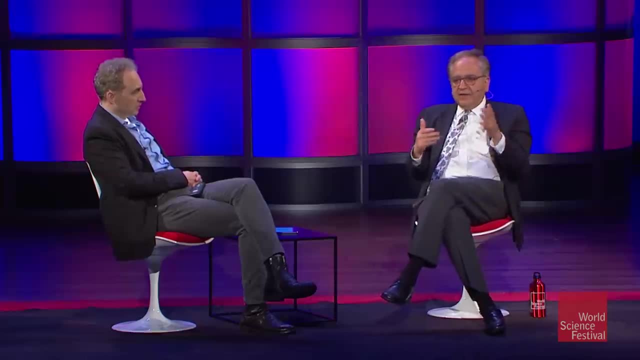 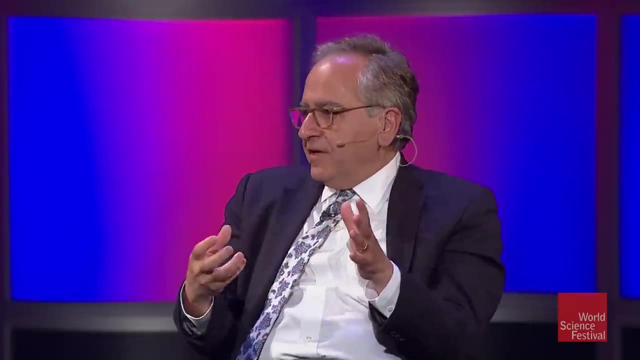 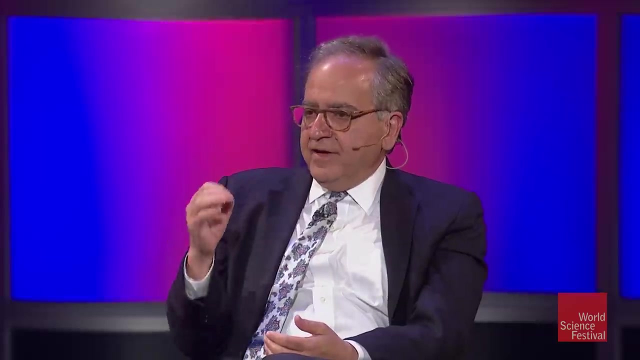 you can lose information. so therefore, indirectly there was a proof that whatever happens to black holes, the information should get out. so that's that part was kind of beginning to be established using these kind of arguments in string theory. but the wrinkle is that even though there's this mathematical proof, 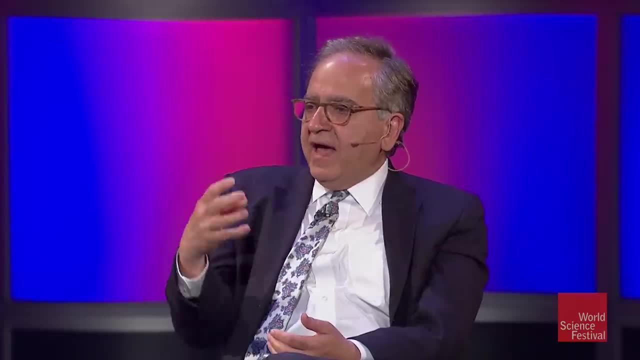 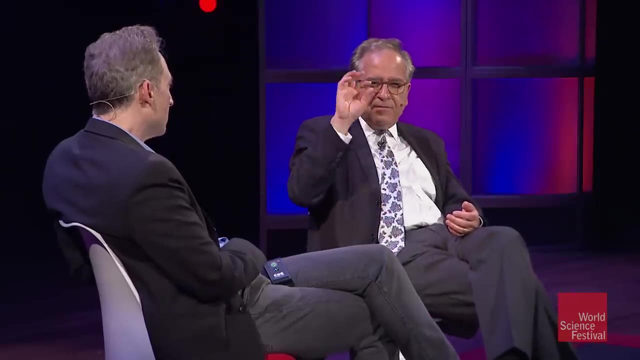 that this should happen. we still did not know exactly how and some people thought maybe the information gets out with this radiation, as you were saying, Brian, very gradually and very tiny bit at a time, but gradually builds up to give you information out. and this is what, in the 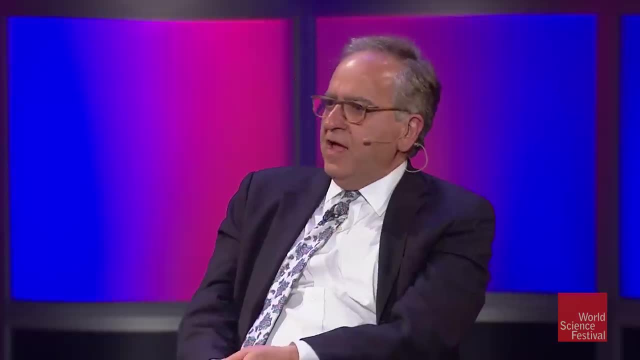 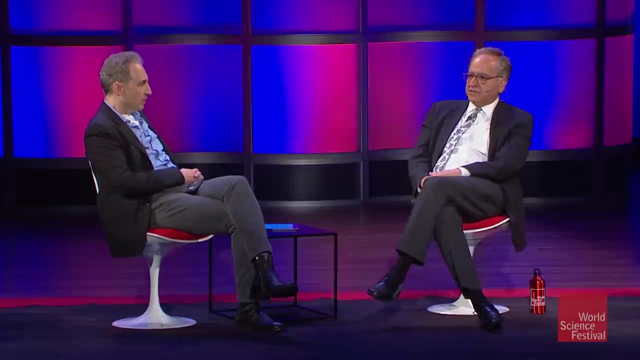 early 2000s, I believe, agreed that this is the resolution, but I still think, and I think the community still believes, we haven't really understood how this happens exactly. so the information puzzle about how this information comes out is still one of the big mysteries of black holes. 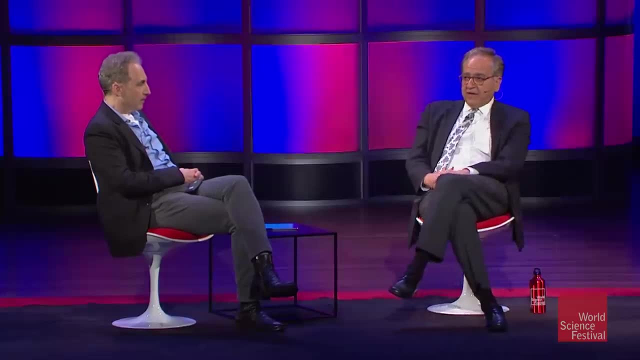 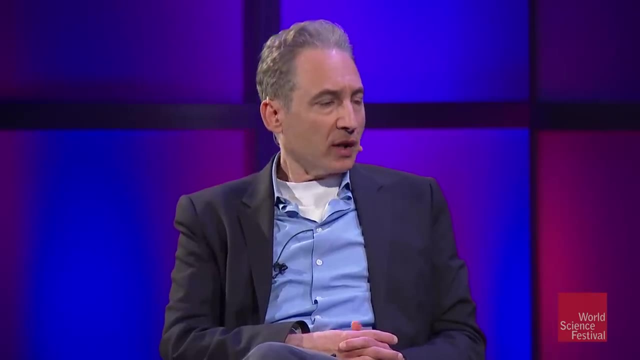 and we don't really understand it. so do you think it's possible that we will one day conclude that the original view of Hawking was right, that the information does not get out? is that still on the table in your view? well, I think it sounds much less likely. 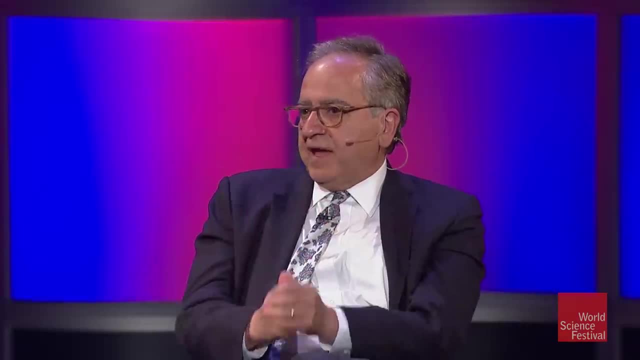 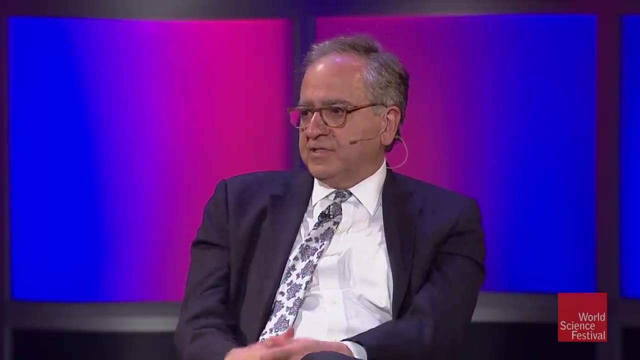 given that we understand a dual description, another description of these black holes. so it seems like that seems much less likely now. but you know, we can never say we know everything about this subject. that's our current understanding. it could of course evolve, but, but even even with that understanding, 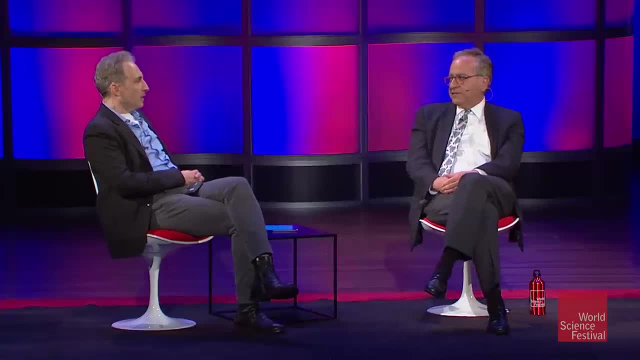 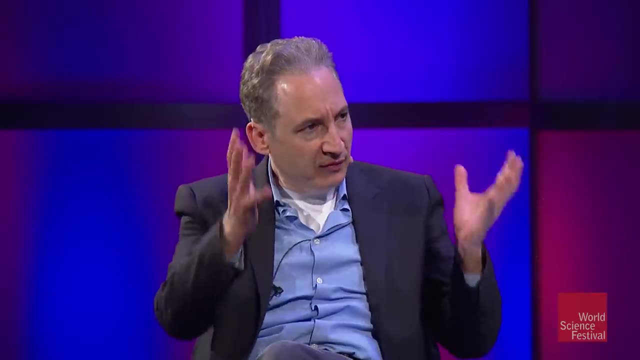 it's not. our understanding is not sufficiently detailed to convince us of this, of how it happens. now, a lot of our discussion here has been focusing on what happens at the edge of a black hole. at the event, it may be information stored. it may be where the entropy 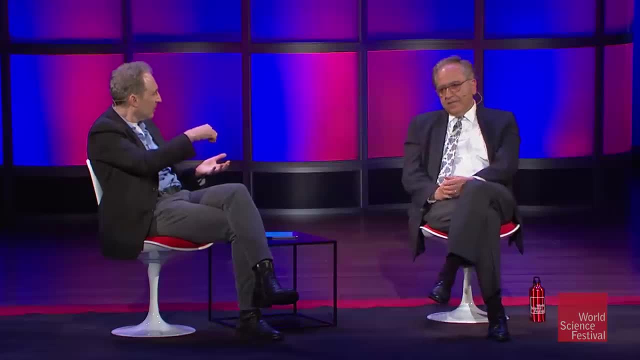 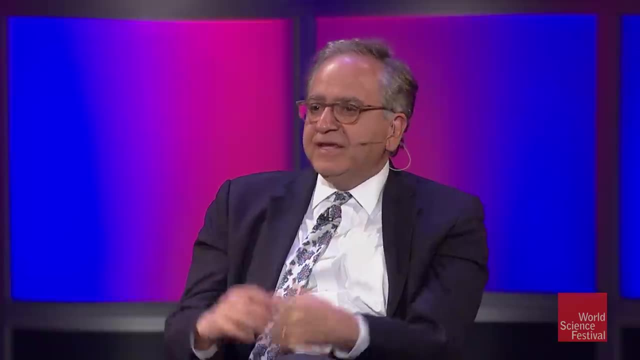 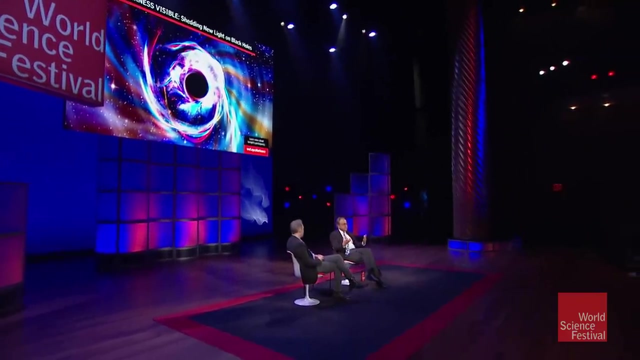 is stored. we haven't said much about what happens at the center, right? can we just spend a little time talking about that? well, one of the things that happens in the center of the black hole is that there is this singularity, this infinity that Brian discussed already. 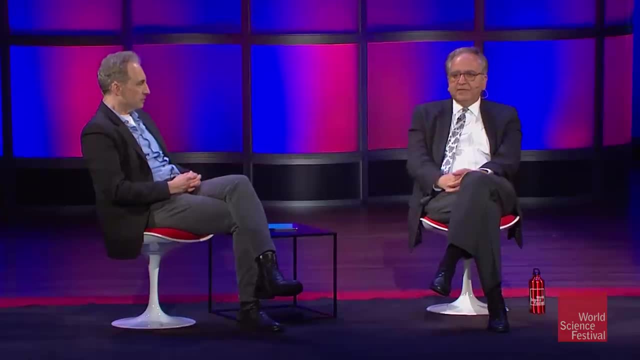 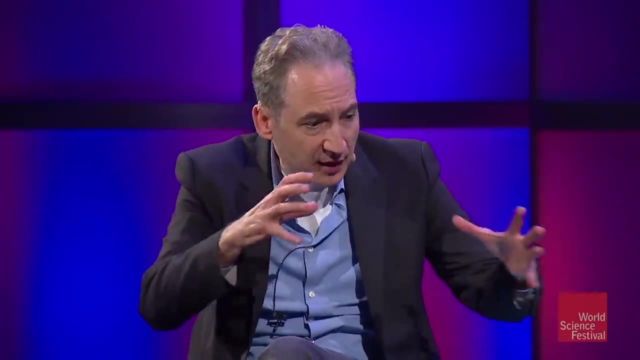 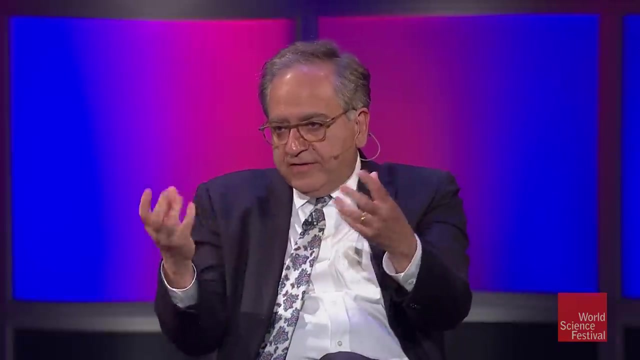 this division by zero analogy, and we don't believe that's physical, we believe that's just the phantom of infinity. now, quickly, the infinity could be physically that you've got all this mass crushed to zero size, and zero size is not physical. for us, there's nothing smaller. 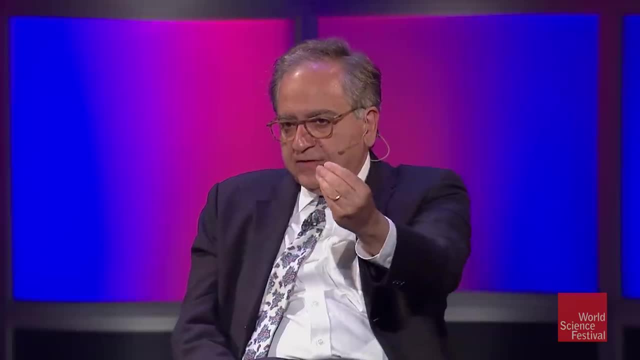 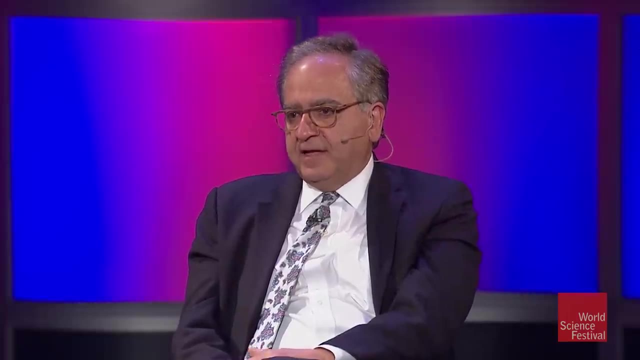 than Planck's length, which is about 10 to the minus 33 centimeters. the notion of space breaks down anything smaller than that, so there cannot be an infinity in physics. we don't believe so, so we don't understand what is happening in that way. 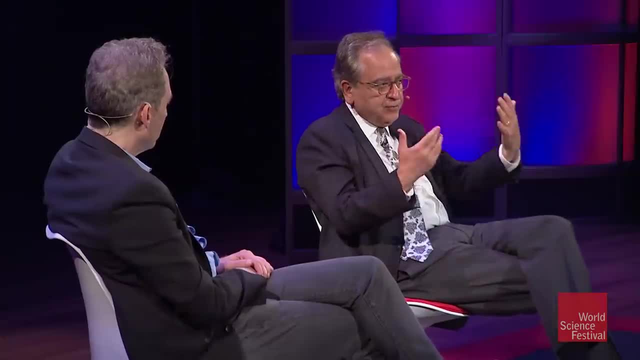 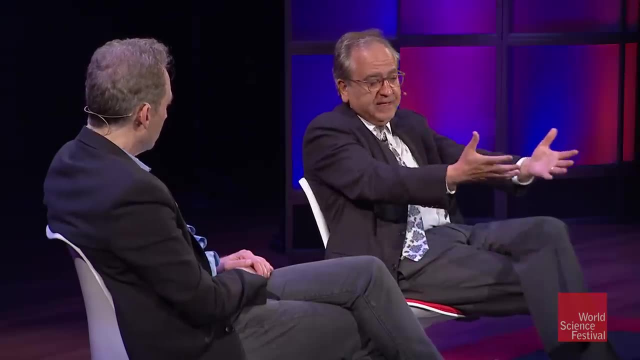 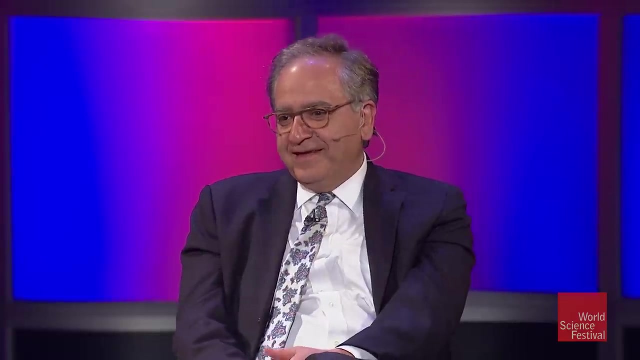 and there's nothing there. we know that there should be a good description, but we don't have it. and why that's important is that, well, we want to know what's happening inside the black holes. of course we can send somebody and find out what happens to that infinity. 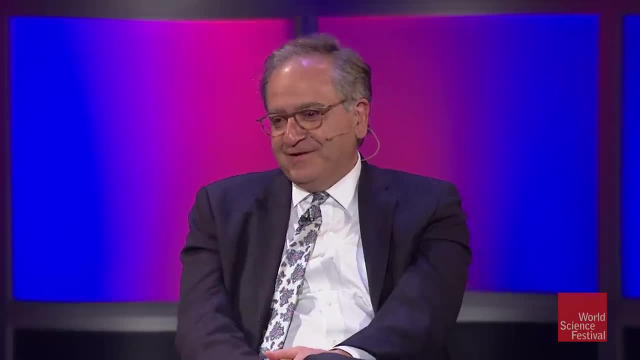 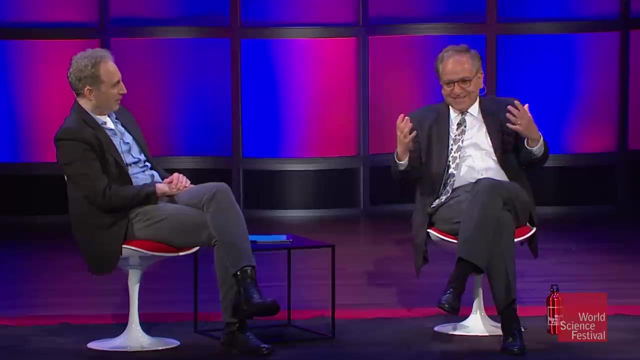 but that would not be a fair thing. and even if we did that, even if we said, well, we send some creature, not us, the robot or something- the robot cannot come back to tell us what happened or what they saw, so it won't be useful. so we have to figure it out. 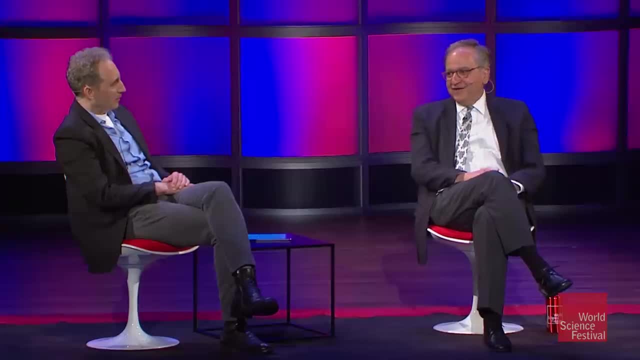 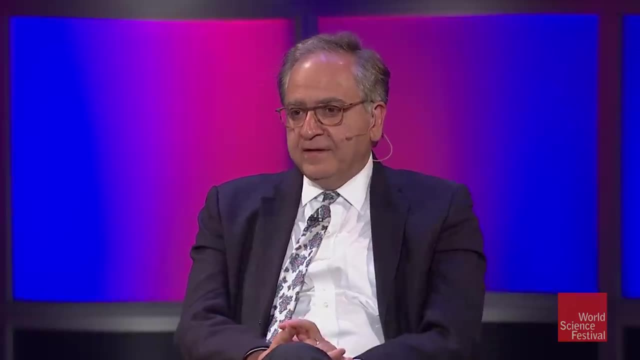 without going inside the black hole. what's going on there? and that's still, we have. no, not only we don't have observational data, we don't have enough theoretical understanding, and we think it's important not just for the black holes, but it turns out that those infinities 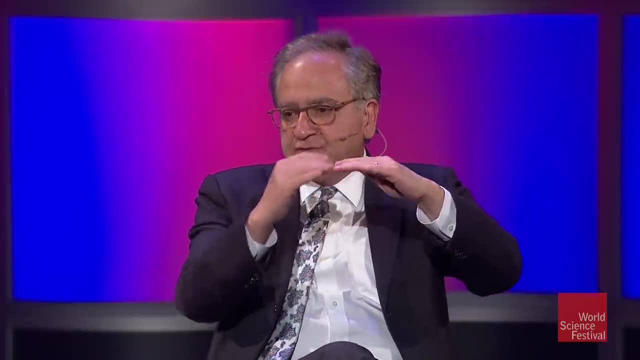 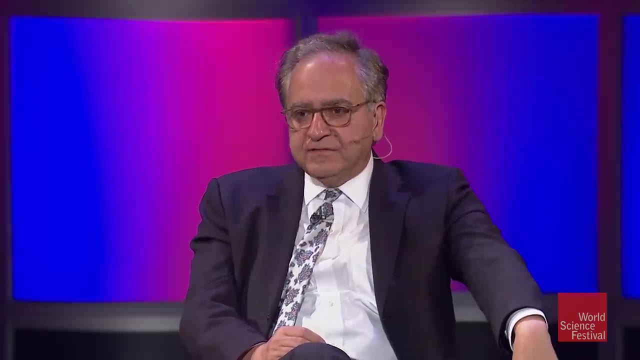 that we see. if you try to pass through those infinities to the other side, so to speak, it turns out. it looks very much like the infinities we see at the beginning of our own universe. it is as if our universe is emerging from inside. 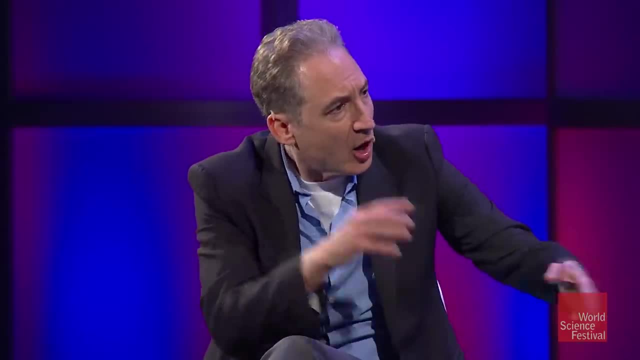 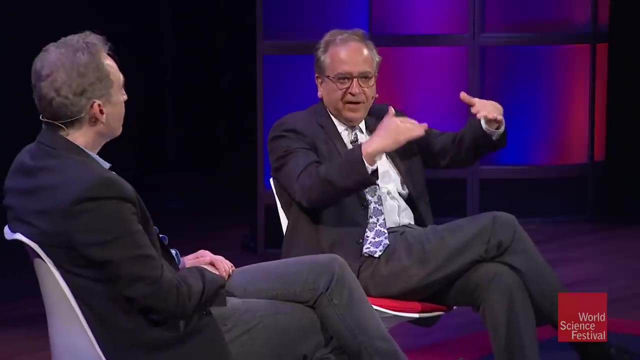 black holes along those lines and don't lose your train of thought there. oftentimes people think of the center of the black hole as a location in space. the center- is that the right way of thinking about it? no, actually it's like in a given time it happens at a given time.